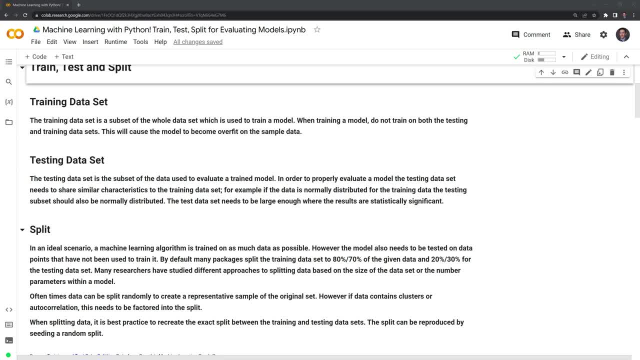 this needs to be factored into the split. When splitting data, it is best practice to recreate the exact split between the training and testing datasets. The split can be reproduced by seeding a random split. Next we'll review the dataset that we have and that we'll use to create. 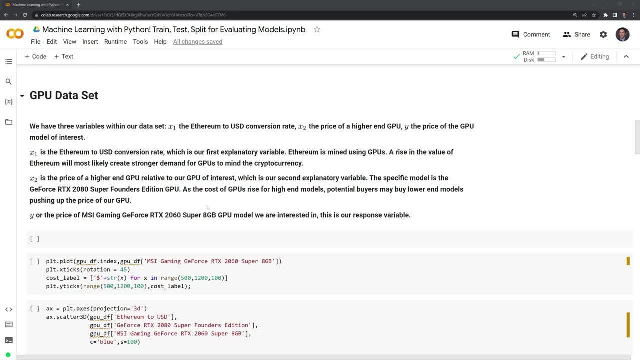 our training and testing dataset. In this case, we have two explanatory variables. The first one is going to be the Ethereum to USD conversion rate. The next explanatory variable is going to be a GPU known as GeForce R2.0.. The next explanatory variable is going to be a GPU. 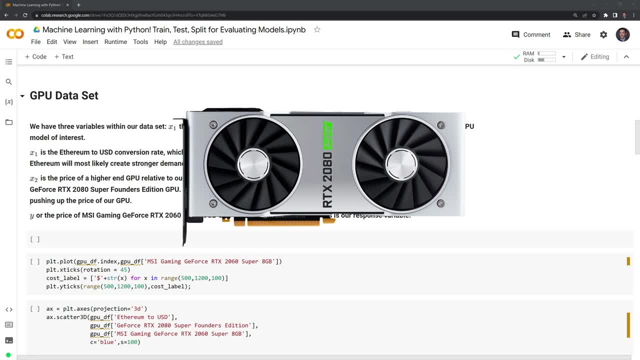 known as GeForce R2.0.. The next explanatory variable is going to be a GPU known as GeForce R2.0.. When 싱 job is Scoop, we wait until theannointed 후 to find out that that GPU lid can be. converted to an oturable ring. When 싱 job is Scoop, we wait until theannointed is destroyed. The nextjamin will differentiated the amount of data allocated by� Where a GB's value on theeraai atérk is 0.8o. Where a GB's value on theeraai ateparate atらetat에şi is the price of thees, knowing that this GPU is worth about $30. where's the data they can be used toward? Where a GB's value on theeraai sprite tánnex is set again? 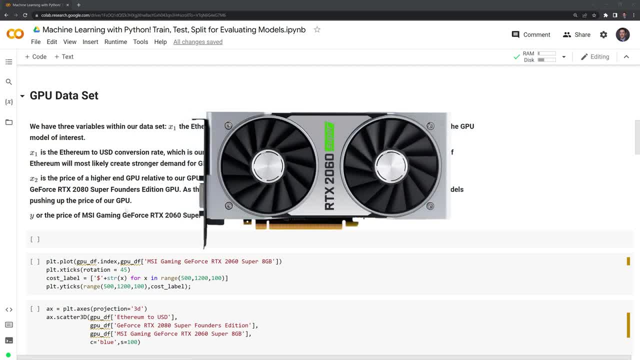 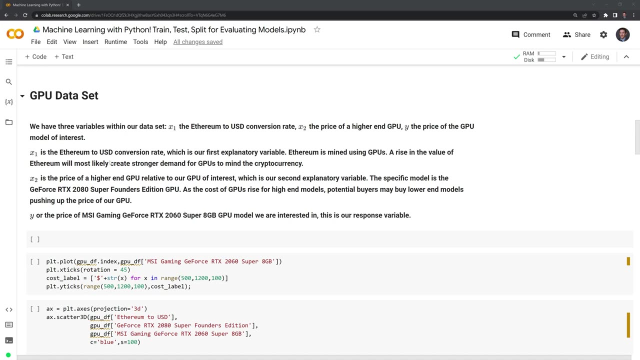 họ are provided an attestation. where's the data? tánnex, tánnex, and there the is a pattern where a GB's value on theeraai solidarity is actually the percentage of data which could happen. GPUs are used to mine Ethereum at this point still, as of May 2022.. 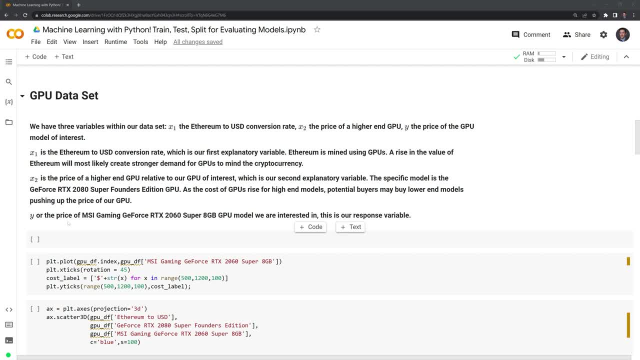 So if Ethereum rises in price, there's going to be more demand for GPUs like this RTX 2060.. Our second explanatory variable is a high-end GPU, And if we have a rise in the price of the high-end GPU, some of the buyers of this GPU might choose to go for a more low-end GPU like our 2060 here. 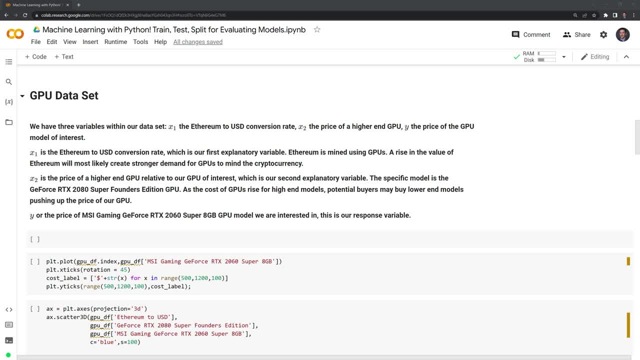 So a rise in this price might also entail a rise in the price of the 2060.. Let's load in our dataset. I am going to load the dataset in using Pandas. I'm going to call it pdreadexcel. I've provided the Excel sheet on GitHub if you want to follow along. 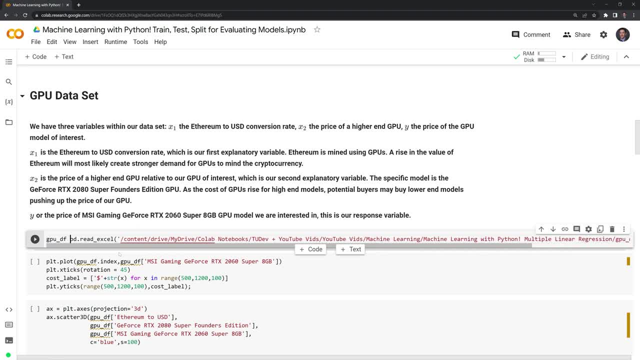 And I'm going to call it pdreadexcel, And I'm going to call this data frame gpudf And I'm also going to set the date column as our index column. So once we have that read in, I also want to take a look at our dataset. 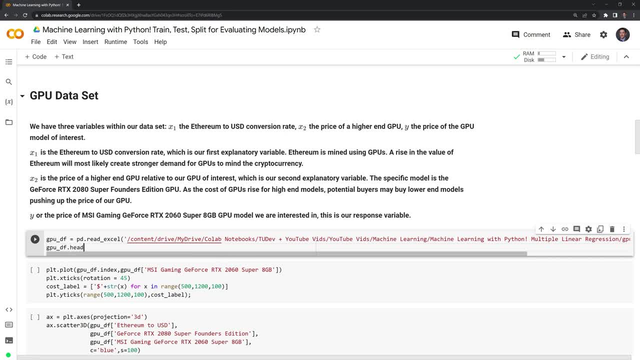 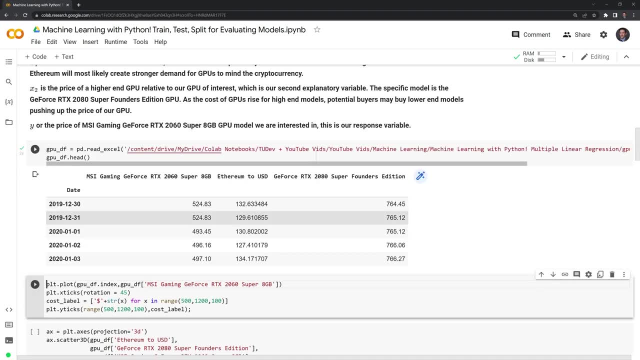 The way that we can do that is we can call the head function to take a look at the first five values of the data. Let's run this And we can see that we have our dataset here. We have our response variable in the first column. That's the price of the. We have the RTX 2060 Super, We have the Ethereum to USD conversion rate And finally, we have the higher-end 2080 Super Founders Edition in the last column here, And the index is the date where all these prices were recorded. 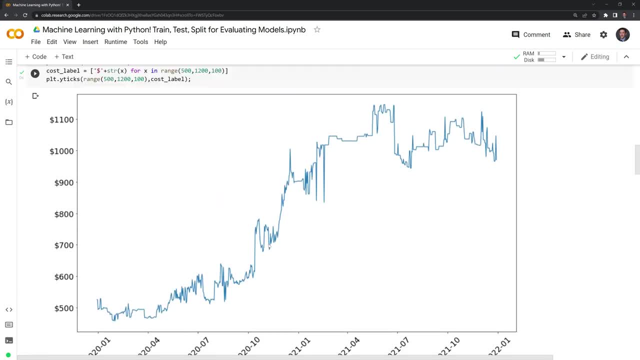 Let's first plot these out and take a look at them, And we have our response variable printed here. So this is the value of the 2060 in dollar terms And we can see that it's Not quite a linear rise in this. 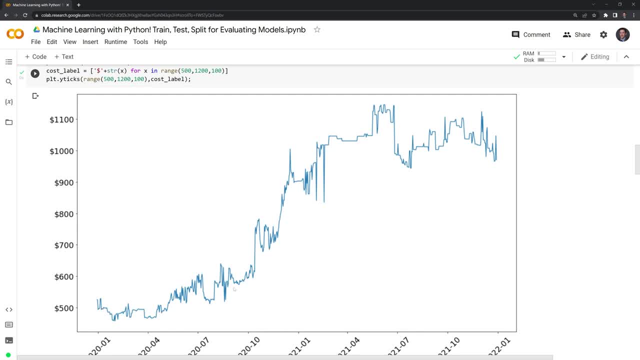 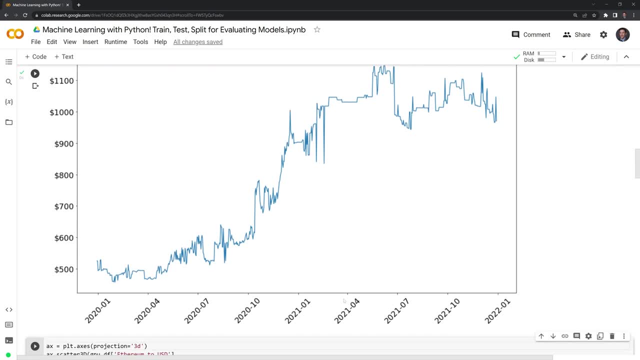 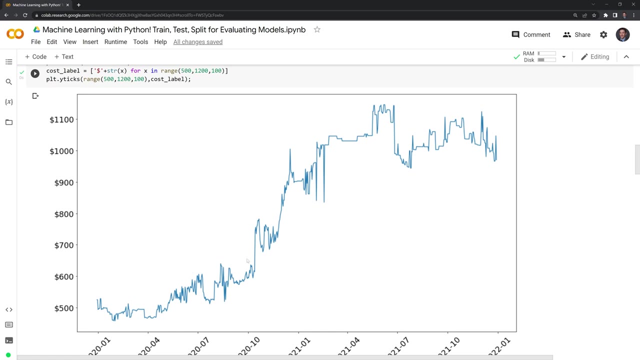 So there's a bit of non-linearity where we have this pretty large spike going from the end of July into the beginning of April of 2021.. So we might want to go with a non-linear algorithm in order to predict the price movement of the GPU. 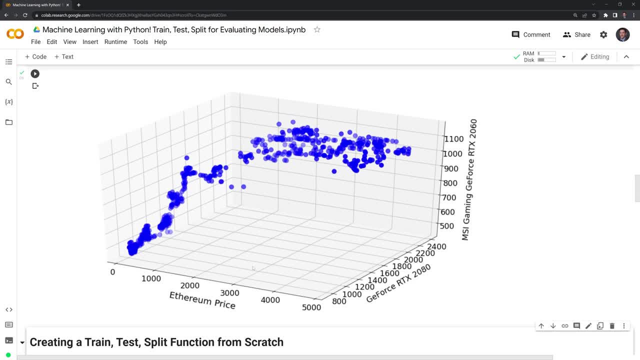 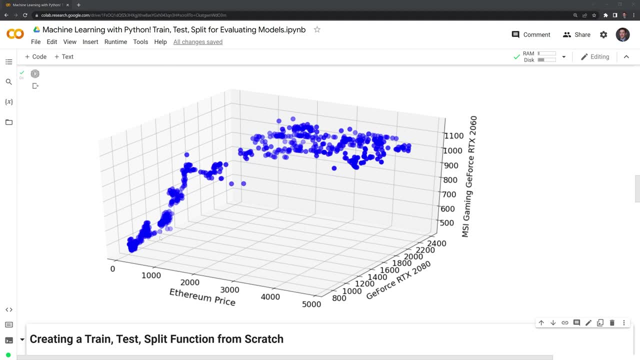 All right. Next, what we'll do is: we're going to, We're going to print out a 3D scatterplot. Right here we have the Ethereum price on the x-axis. On the y-axis, we have the GeForce RTX 2080.. 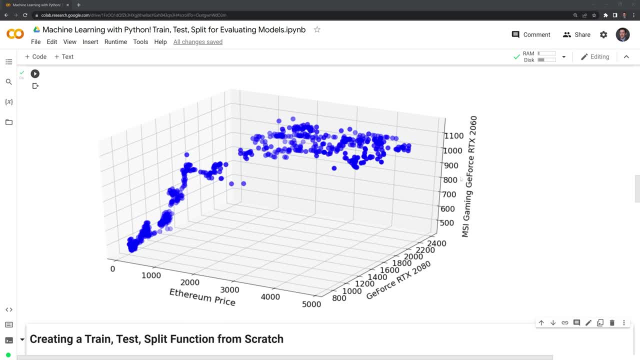 That's the more higher-end GPU. And finally, we have our response variable on the z-axis And we can see here that we still have that non-linearity. So when we go to figure out the type of model we'll use, we'll have to factor that out. 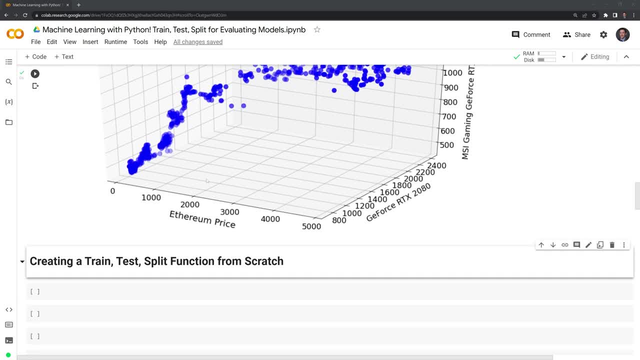 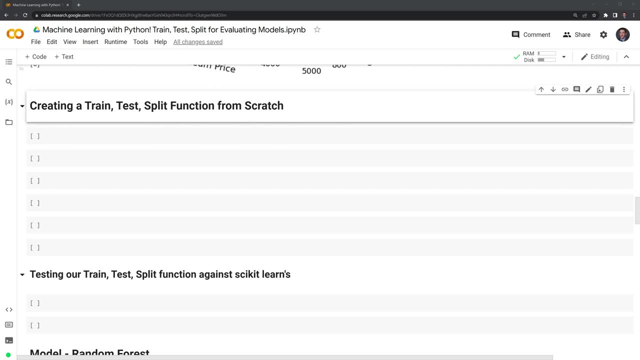 And we'll have to find out where is that going And we can use that into our modeling. What we'll do first is we're going to create a train test split function from scratch, And then later on we'll take a look at scikit-learns train's test split function as well. 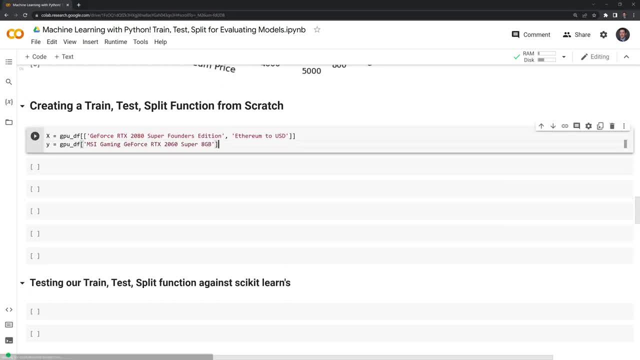 What I'm going to do first is I am going to load, create two variables. The first is going to be x and it's going to contain the values for the 2080 Super Founders Edition in Ethereum, a panda series of the response variable, And the way that we do this is we just call the GPU data. 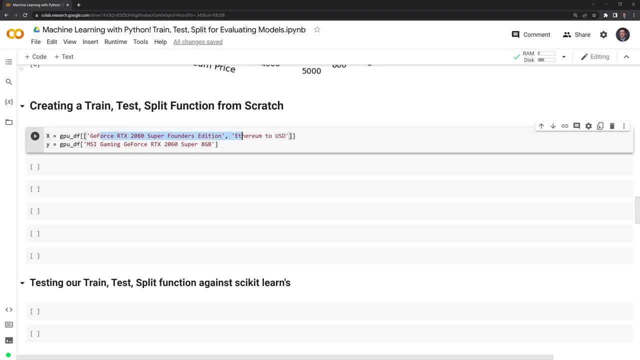 frame And then, within two brackets, we can create a data frame containing just these two. And then here this will just be a data series, a pandas series, by just calling this column here. So let's run this And let's get started on actually creating our function. So what I'll? 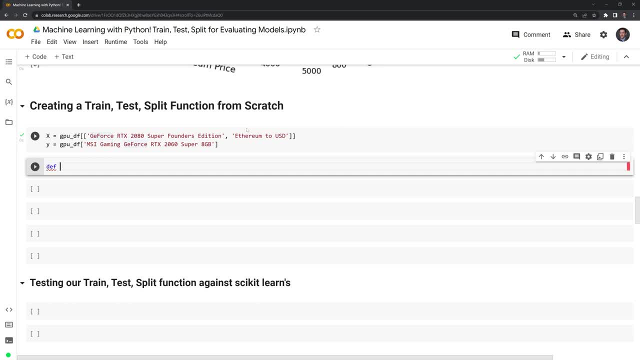 do first is, since I'm creating a function, I need to start with depth, to define it, And then I'll call our function TTS, So train test split. In this case, I am going to if the function is going to need a few parameters- x values, y values- So this is going to be our. 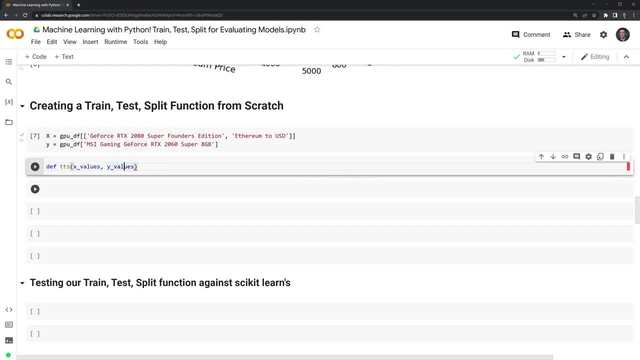 explanatory variable here And then response variable is the Y variables. We also need our need the test size. So this is going to be the size of our testing data set By default. I'm going to set it to 25%, right in between the 20 and 30% I stated before. And also we need to put 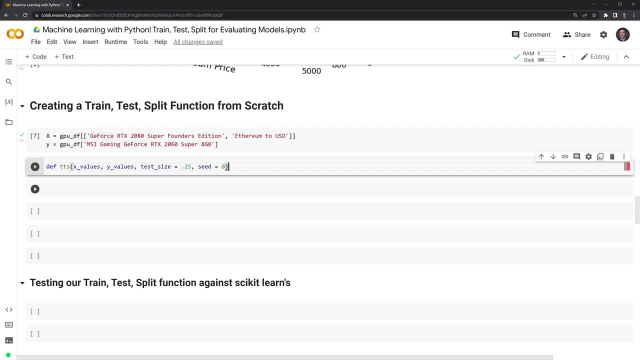 in a seed, because we are going to split this randomly And we want to be able to recreate this. Like I said, it's good practice to save to be able to recreate any random splits that you make. So what I'm going to do is I'm going to create a try and accept, And I'll explain this. 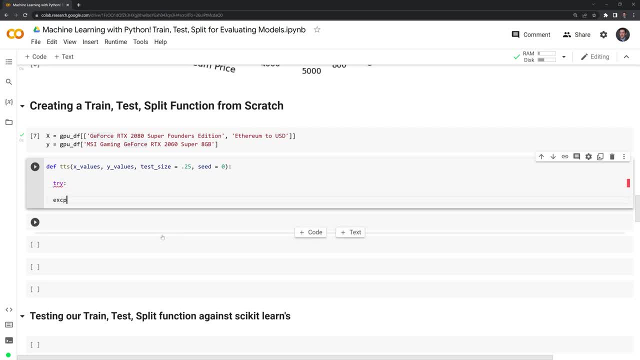 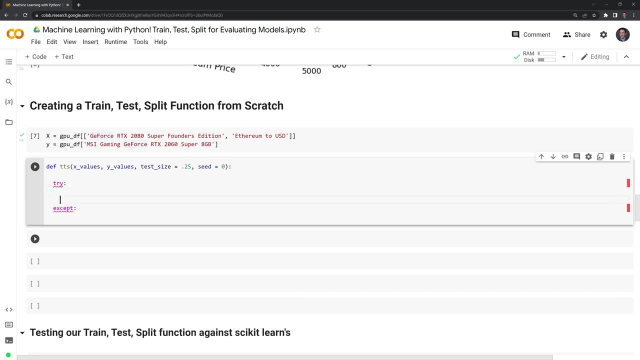 later why I'm doing this. But I'm going to first create, go through the try and then I'll explain the accept. And what I'm going to say first is, depending on the type of instance, we're going to create, an if else statement. So just to explain this here, I'm going to say if is instance And 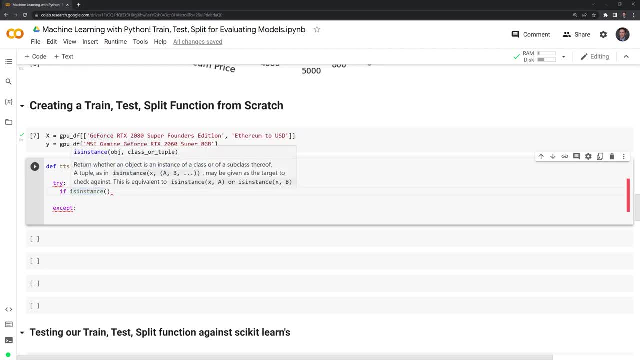 this built in function is instance can test the type of data being input, And in this case I want to say if a pandas data frame or a panda series is input. we want to do this, But we first need to check that it is. so I'm going to say x values and then comma, and then I want to say if the x values. 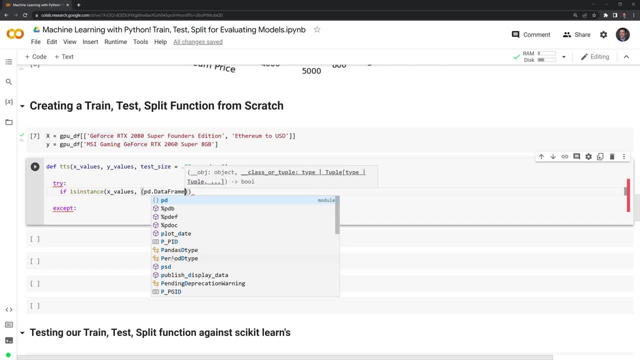 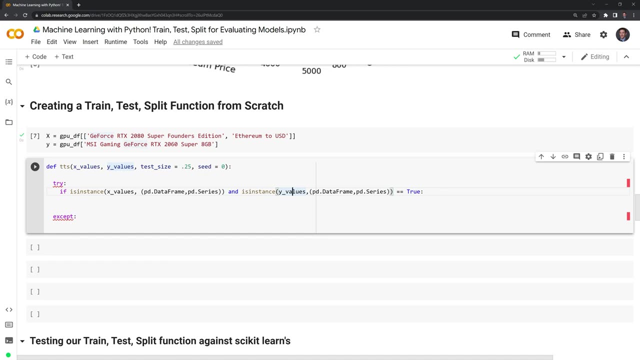 input is either a data frame or if it's a panda series, then I want to go forward with the if else statement, with the if statement here, And I want to do the same thing with the vibe y values, And I'm going to have this. and so if both of these are true, then the code below is going to: 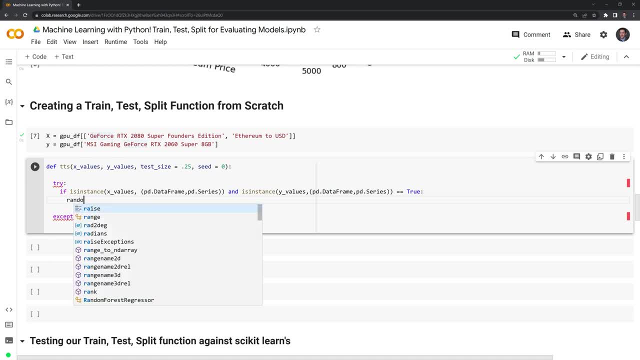 be executed. What we'll do is we're going to create a another data frame And in this case we'll call this random DF for random data frame, And what we'll do is we'll call the pandas- can cat function? and this is going to. 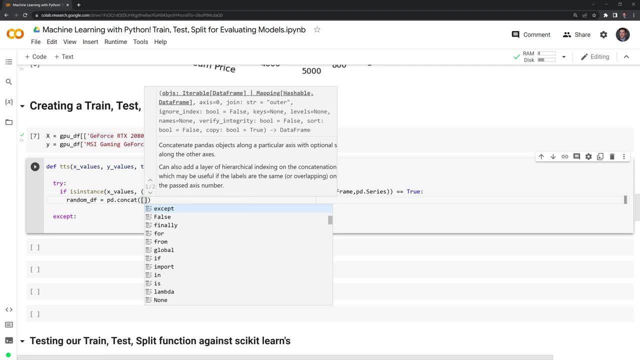 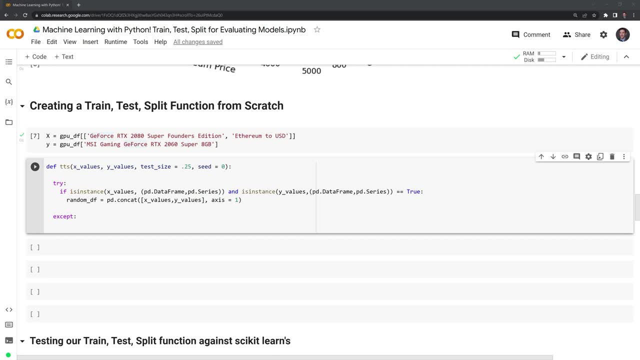 combine our x and y values together And I want to set the axis is equal to one, So we combine it and we join it together left and right And we don't just append the data to the bottom. What I'm also going to do is I'm going to call the sample function. This is a built in function. 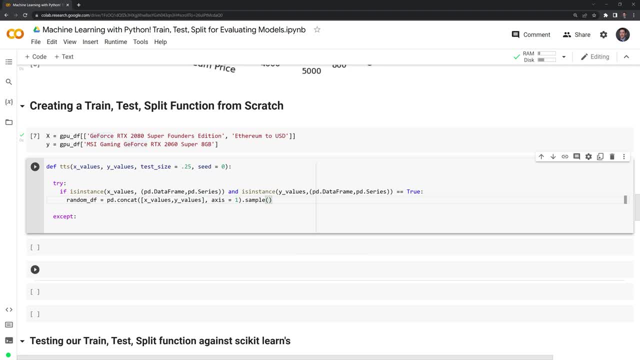 that randomly resamples the data, And this is where the where randomizes the data for us to see what happens. And what I'll say is: fraction is equal to one. So we want to still keep all the data, we just want to reshuffle it. And then I want to also set in the random state, and I am 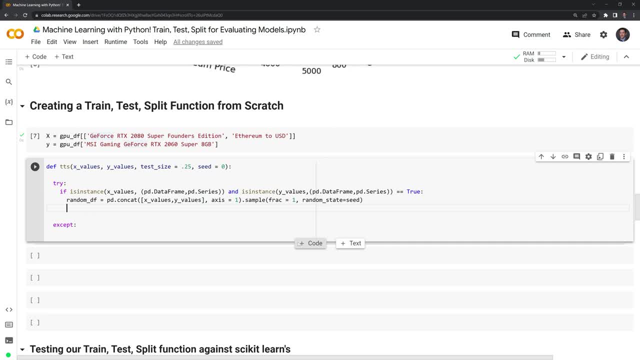 going to feed it the seed that we defined earlier. Next, I am going to also slice the value, or create a slice value, And what this is is it's going to be equal to the total size of the testing data set. So if we have, for instance, we can also highlight this here, if I copy: 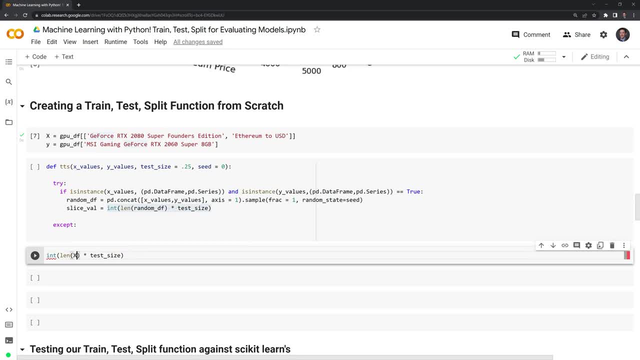 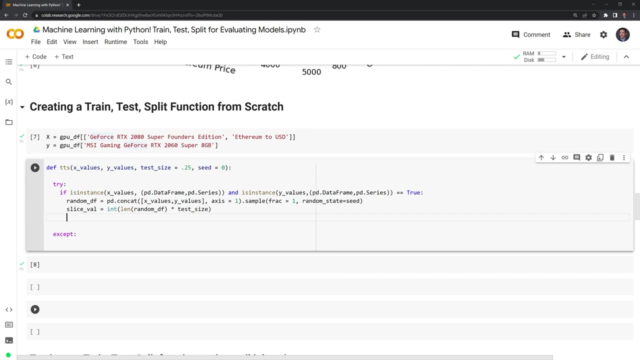 this, and if I just switch this out for x multiplied by point 25, then if for our testing data set we want 182 values, that's going to be 25% of the data given into the TTS function. Next, I'm actually going to create the test data frame and the train data frame And we'll 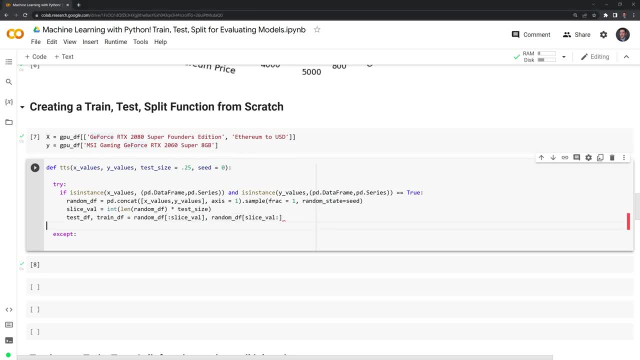 use that slice value in order to create the testing data frame first. So if I do this over here, I can say, just to give an example of GPU DF, same thing that I did before: 128.. So this gets 100.. This gets. 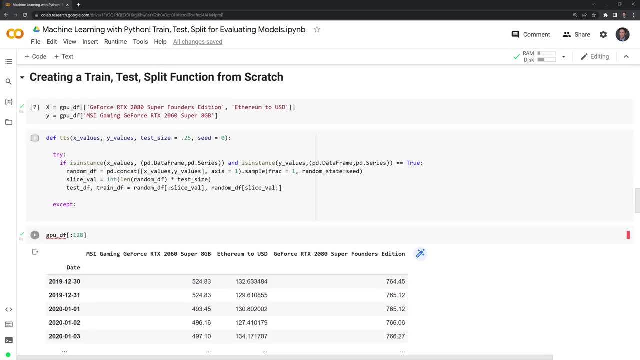 us a data frame of 128 data points. that's going to be the testing data set. then the trading data set is going to create the or we create the training data set by, instead of having the value, the slice value on the right hand side of the semicolon we have. 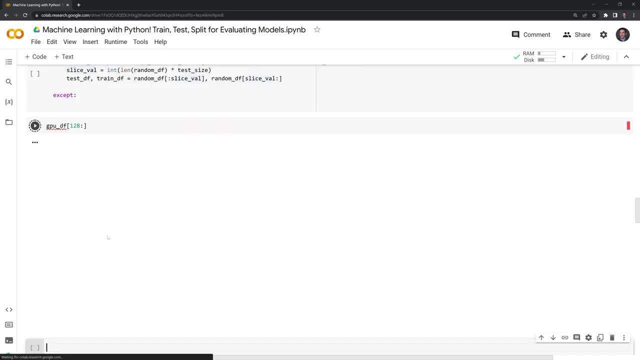 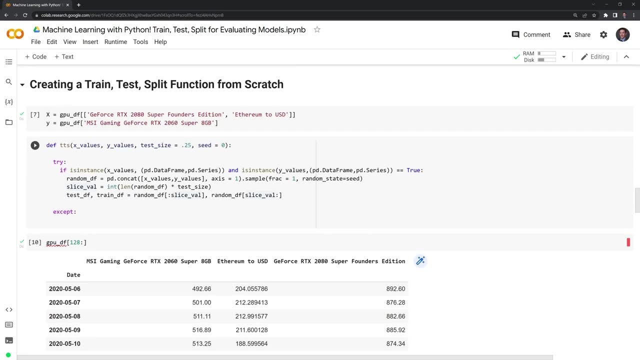 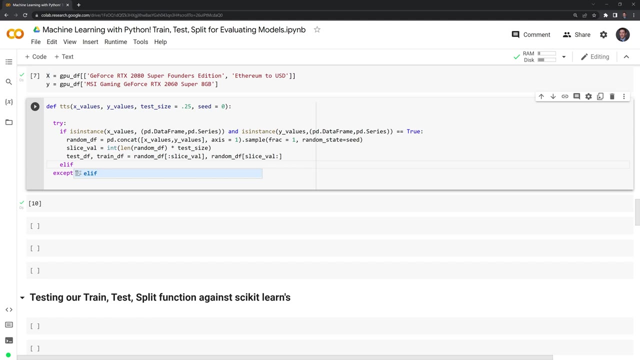 it on the left hand side. So if we take a look here, run this for 128.. This time we have 603 values And we need to add six hits at the endpoint value And that's going to be saved into each of these data frames. 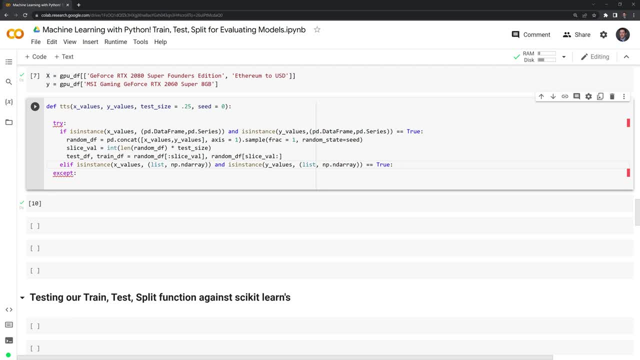 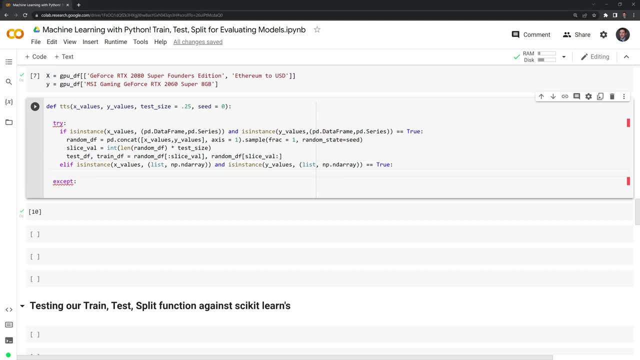 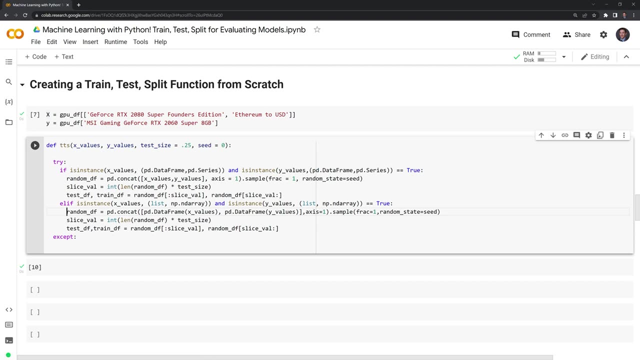 values as a nested list and the y values as a nested list. this function will be able to go through and do the same thing here, And we'll still create our random data frame here. The only difference is we need to explicitly put the x values and the y values into a pandas data. 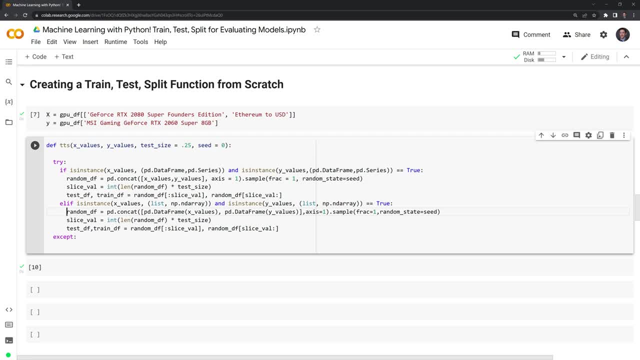 frame, but we'll still concatenate those two together and then resample it, so we randomize the testing and training data sets. Finally, my except is going to print out: if the x values and y values aren't in the same data type, then make sure that they're converted. 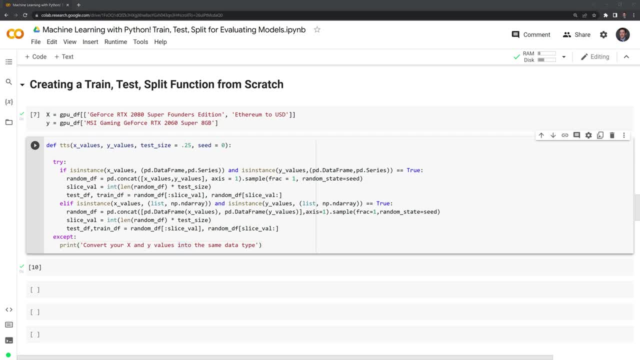 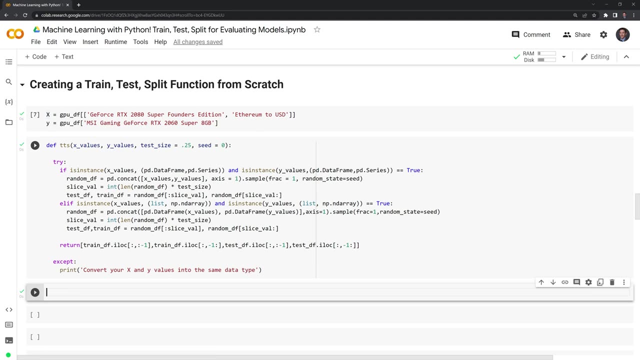 into it And I'll show an example of this later. I also want to actually return the x train, y train, x test, y test values. So we'll return it on the outside of the if state frame in here. Let's run this And then let's test it out. So we have our x and our y values. 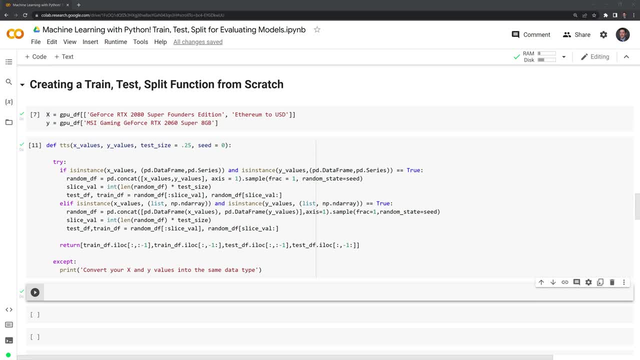 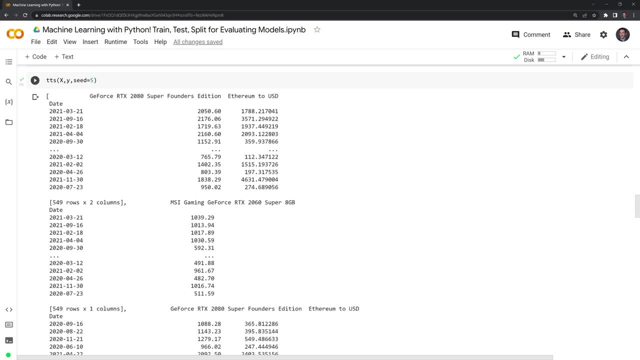 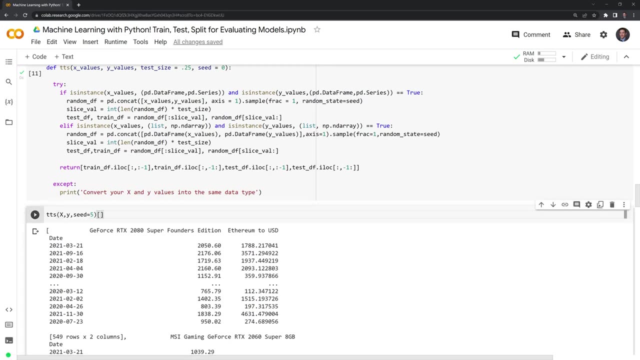 What I'll do is I am going to run the function. for that, I'll say that the seed is equal to five. Let's see Great. So it looks like we have four different data sets here, If, for instance, I take a look at the first data frame in here. 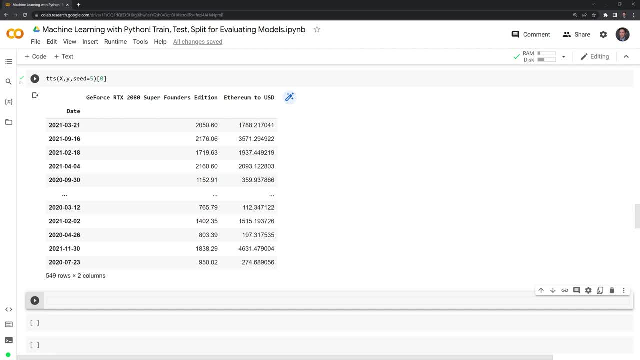 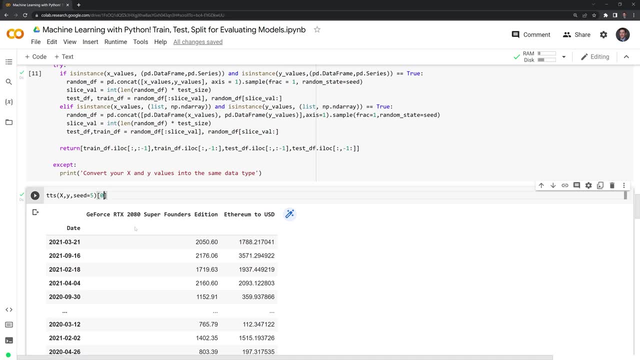 This is our training data frame And we can see that there is 549 data points or 549 rows for this data frame, And this is these are the x values. If I want to see the y values or the x values for the testing data set, I can go to index position. Actually, it'll. 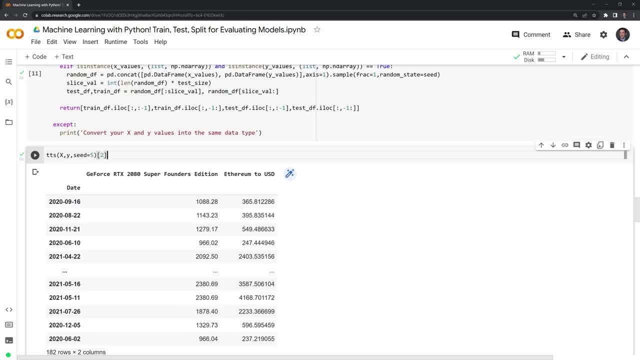 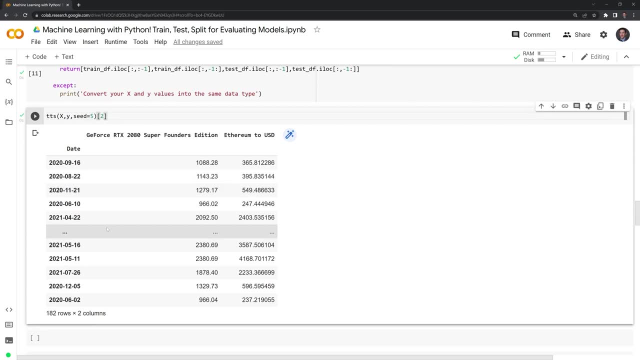 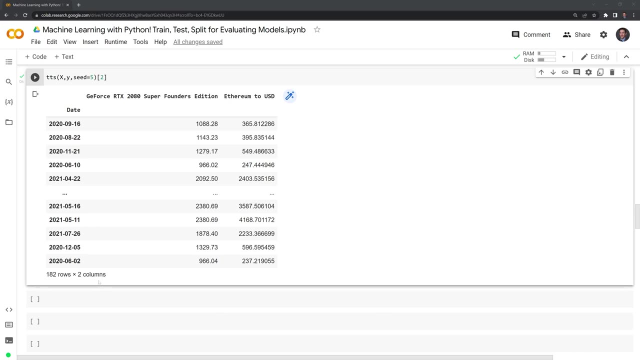 be index position to run that And we can see that we have our explanatory variables for the testing data set here And what we could do also is we can check that this works with our NumPy values. The way that we can get NumPy values is if I do, for instance, x dot values, that returns. 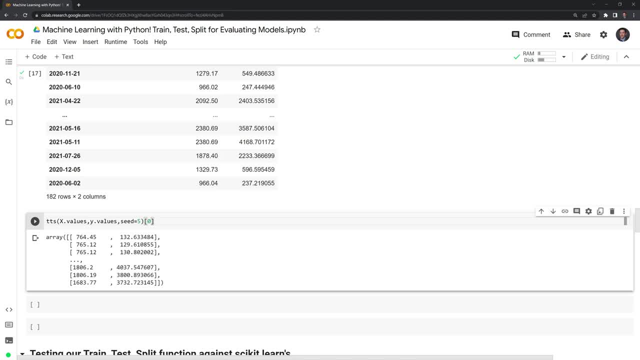 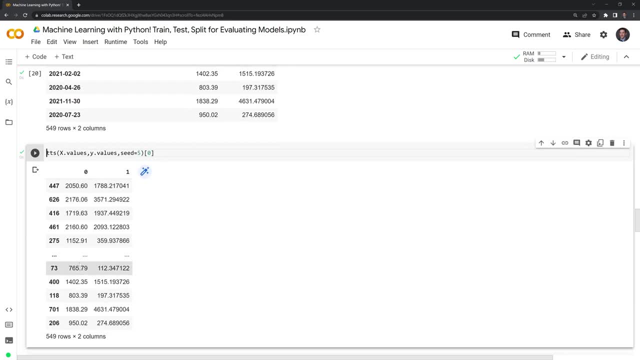 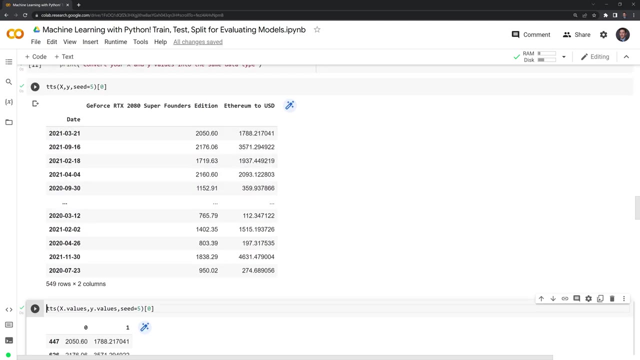 NumPy arrays, So I'll just run it to make sure that we have the same values here. Let's go back up here, set this to zero And it looks like it was the same, given the seed of five. The only downside is the dates are no longer saved and neither are the column values. 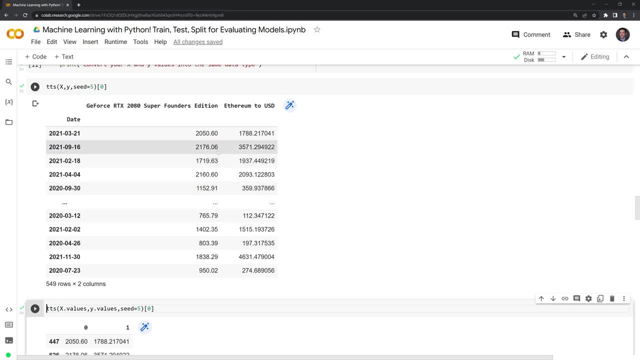 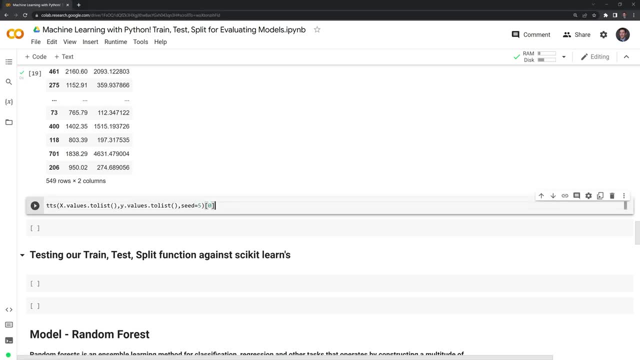 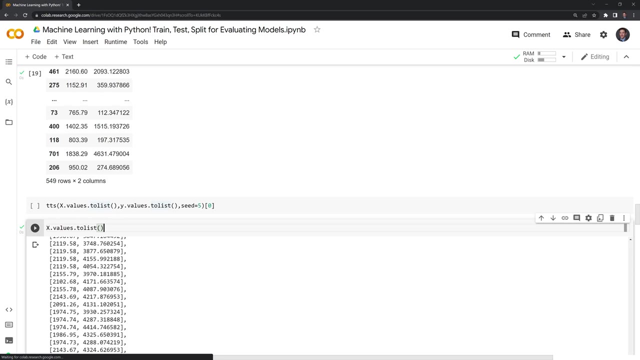 So it's probably best to keep it as a pandas data frame or data series. We can also test that it works for a nested list. The way that we can get a nested list is we can go from a NumPy array to a list And we have a nested list. So let's try running our function on. 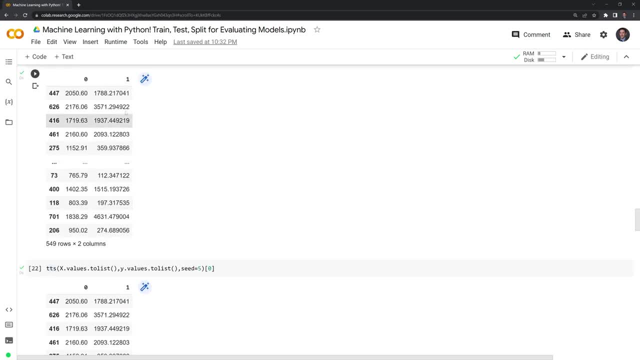 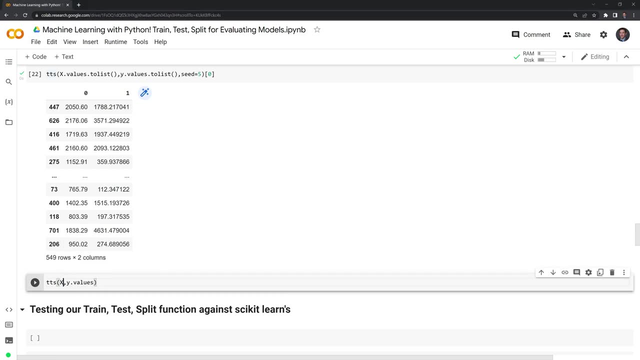 that Okay, And it looks like it was able to run that successfully. Finally, what we'll try to do is we're going to try to use a put in a pandas data frame for the x values and then a NumPy array, And we'll get that message right here once we run this. So let's try. 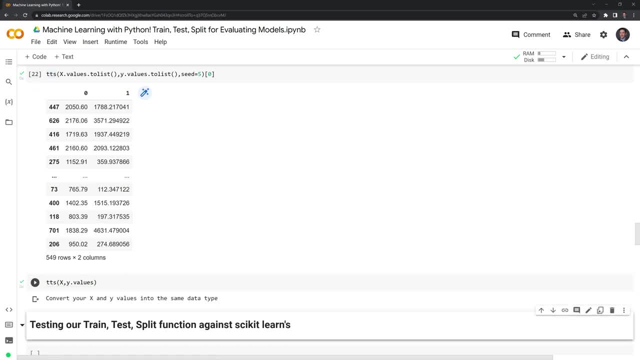 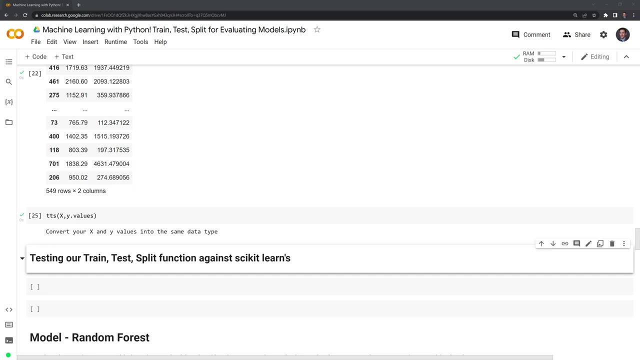 this out And it's telling me to convert my x- y values to the same value. So if I just change this to a pandas data frame, it will work. What we could do is we can test how well our function works in terms. 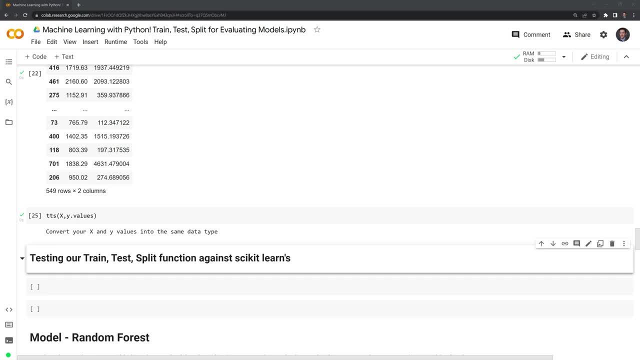 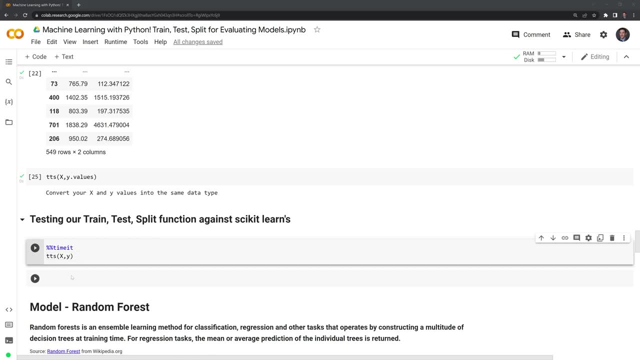 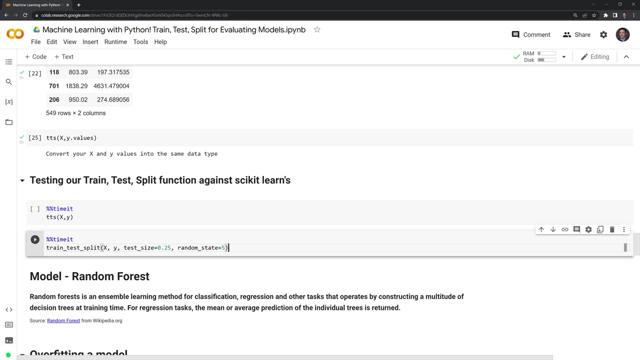 of how quickly it can run relative to the train test split function from scikit learn. So I'll use time it to test my function that I created from scratch, And we'll also test the train test split using the same exact variables here the x, y, same test size. 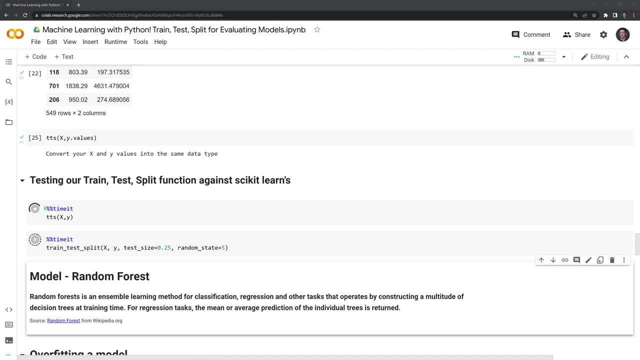 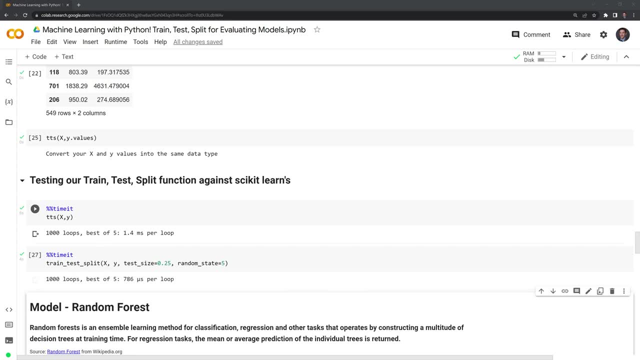 and same random state. Let's run these. We can see here that scikit learns train test split function is quicker than the one I built here. It's only 786 nanoseconds, while the one I created is 1.4 microseconds. So the 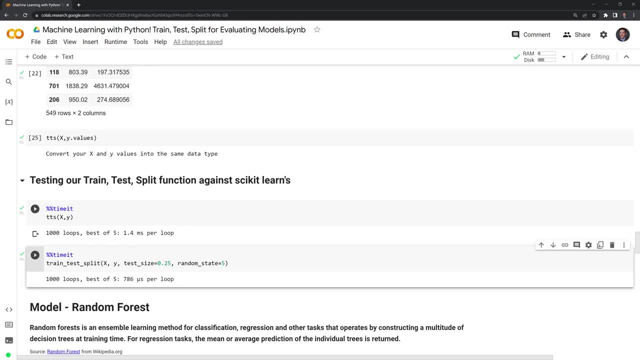 train test split is roughly twice as fast relative to the one I created, So we'll just use the train test split function from scikit-learn, But now that we coded it out by hand, we have a better idea of how the train test split. 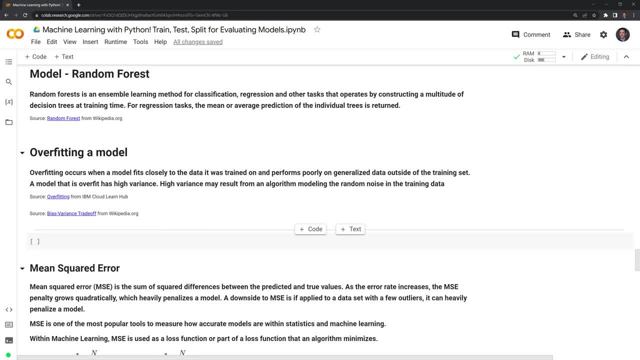 function works. Like I said before, we saw that the data seemed to be nonlinear, So we can use a random forest in order to try to model the data, And random forests is an ensemble learning method for classification, regression and other tasks that operate by constructing a multitude of 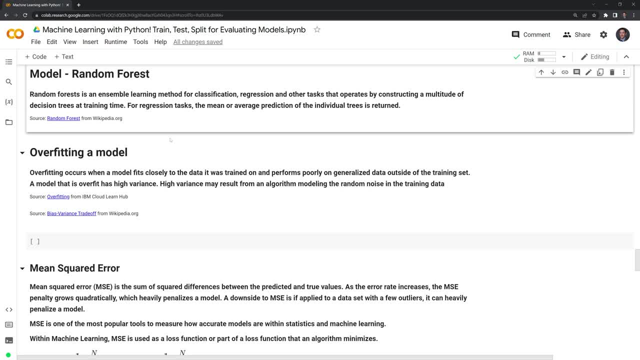 decision trees at training time. Finally, for regression tasks, the mean or average prediction of the individual trees is returned. So in our case, since we're trying to forecast the price, we're going to use a random forest regression rather than a random forest classification. 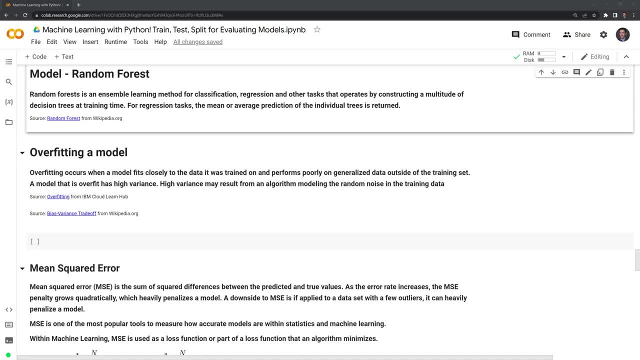 And what we'll do first is we're going to take a look at how overfitting works. So overfitting occurs when a model fits closely to the data it was trained on and performs poorly on a generalized data outside of the training data set. A model that is overfit has high variance. 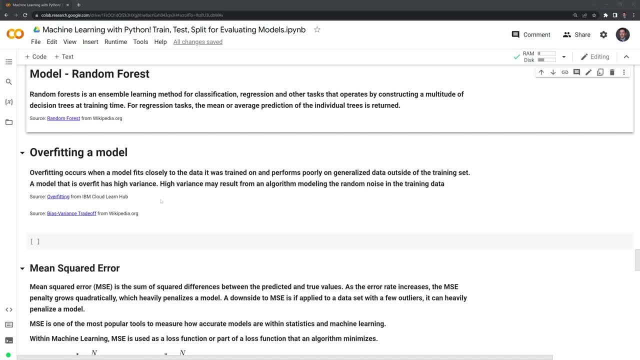 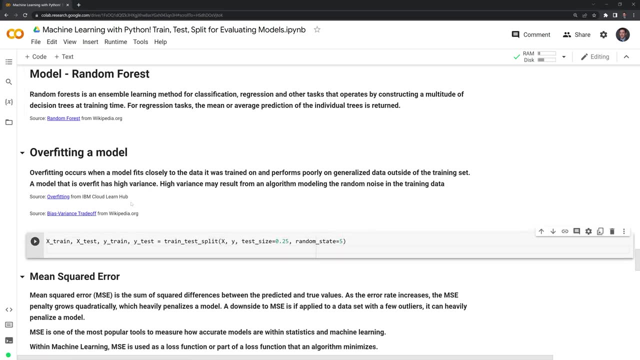 High variance may result from an algorithm modeling the random noise in the training data. What I'm going to do first is I am going to save my variables for X train, X test, Y train and Y test, And if you've ever looked at code from scikit-learn, you've probably seen it this way. 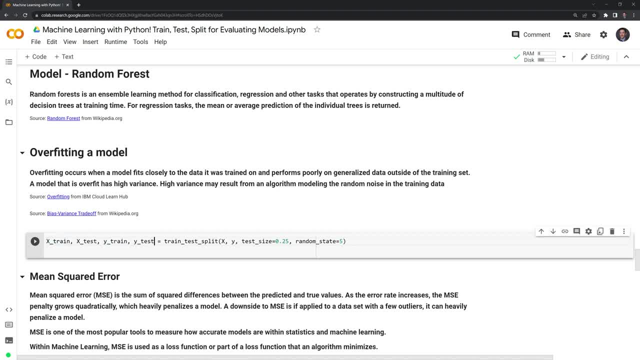 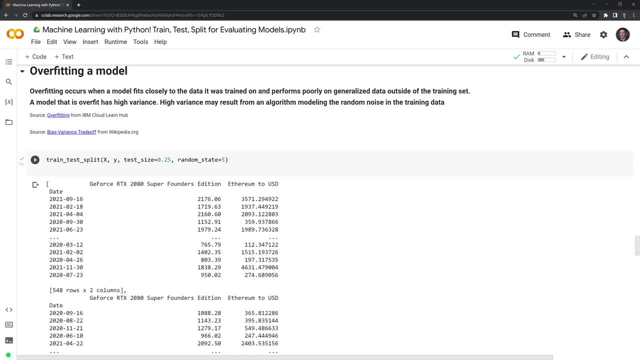 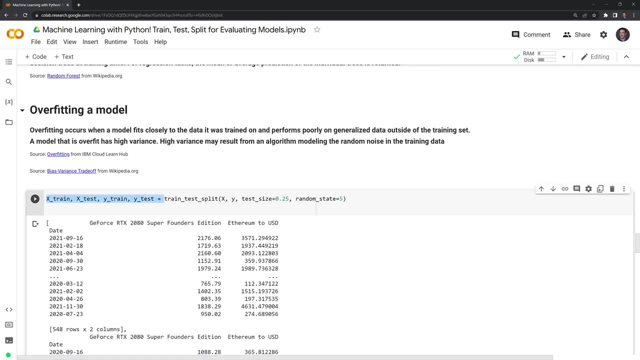 So we can define our first four variables from the train test split method for scikit-learn. So if we just run the method before saving it, we can see that we still have this list here, like we created before. So we have our four variables defined here And we're going to 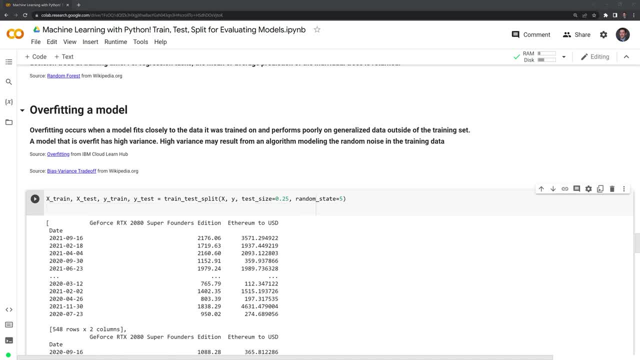 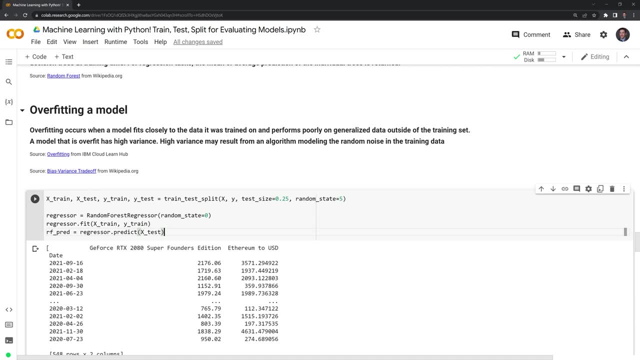 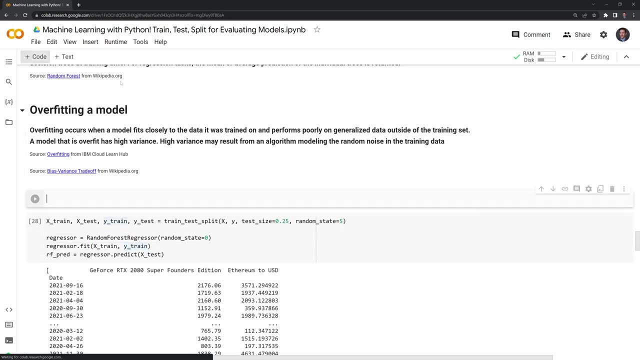 split the data first And then we're going to next fit and predict the data And we're going to train the data on the X train and the Y train data set. So if we take a look at the X train and Y train real quick- we can take a look first at the X train- We can see that we 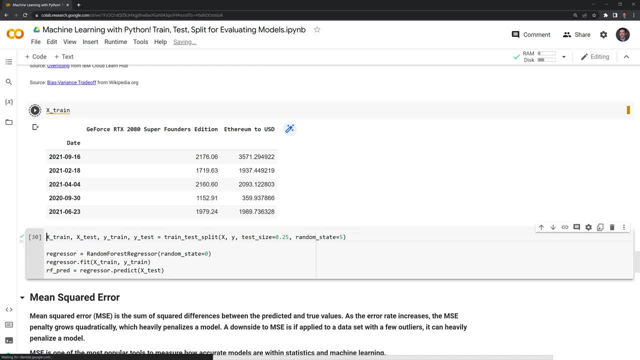 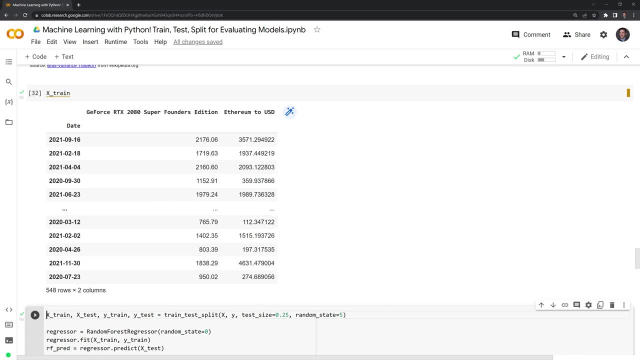 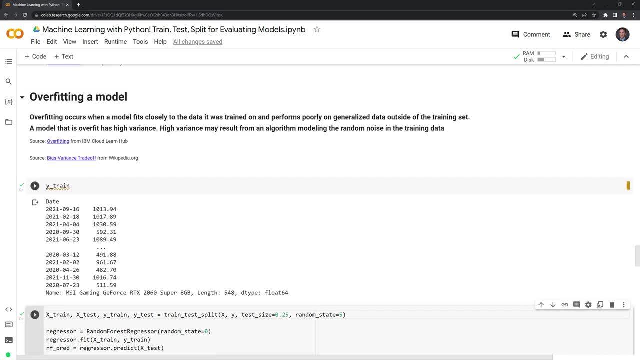 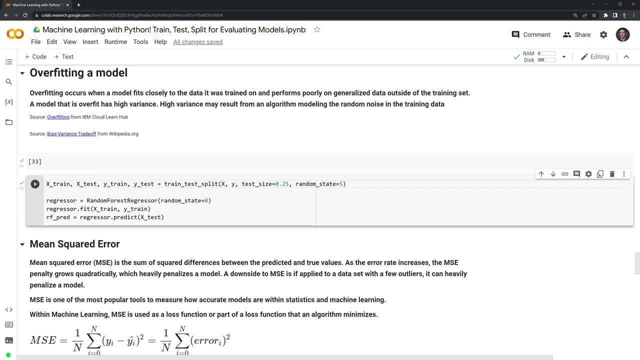 have our explanatory variables, And this is just a portion of it. So it's split by 25% of the data, or sorry, 75% of the data is the training data. Then we're fitting it And then we're predicting the X test value. So if I take a look at the X test, 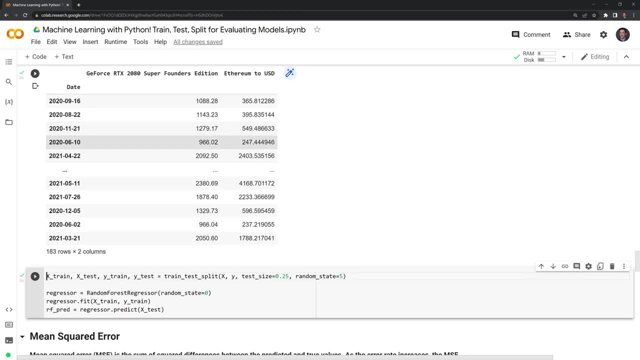 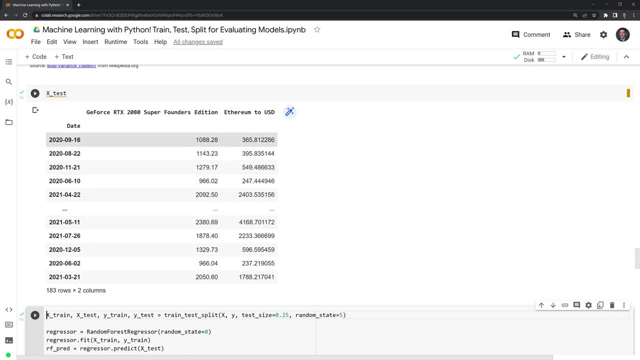 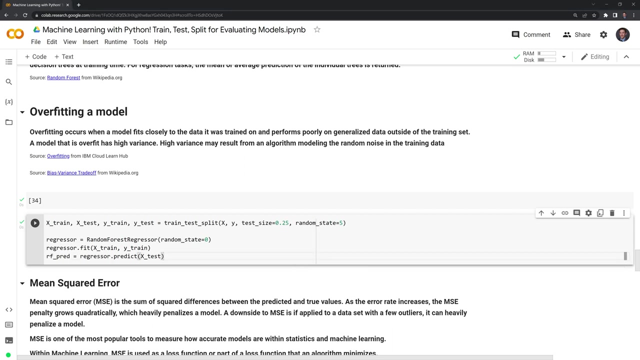 values. that's going to be the other 25% of the data, which is now the testing data. Based on these values, our random forest regression is going to take each of these inputs and predict the value of our 2060. GPU price. What we'll also do is we're going to create a model that's overfit And in this case, 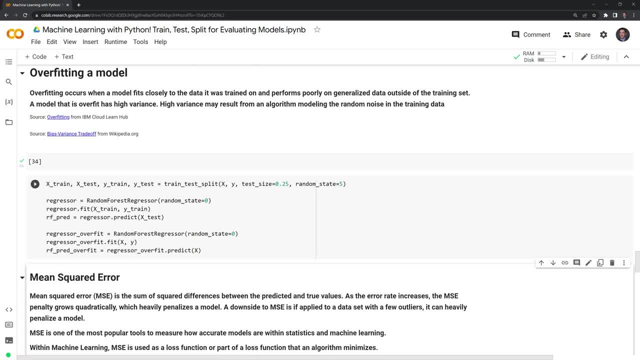 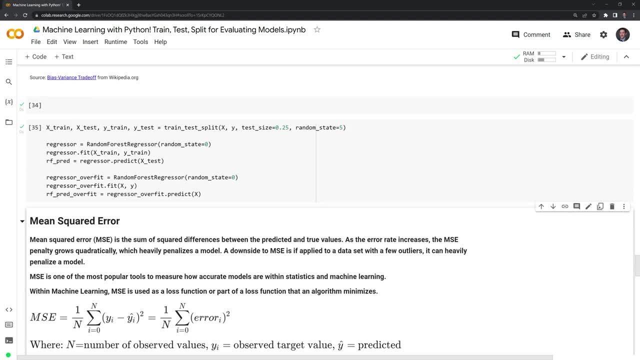 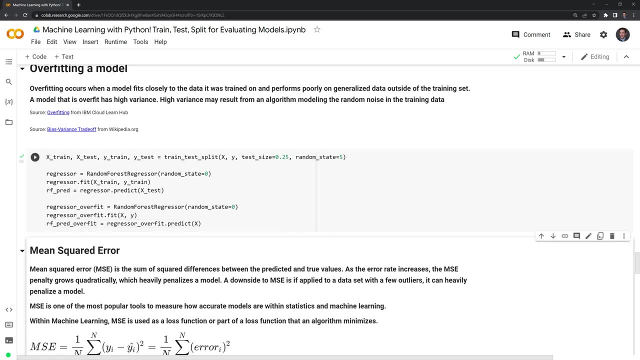 instead of training it on the X train and Y train, we're going to train it on the whole data set, And this is going to cause overfitting. So we'll run this And then we'll move on to testing the each of these models: the overfit model and then the model that was split- 75%. 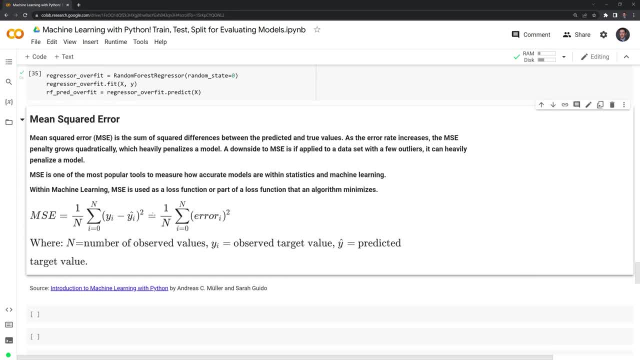 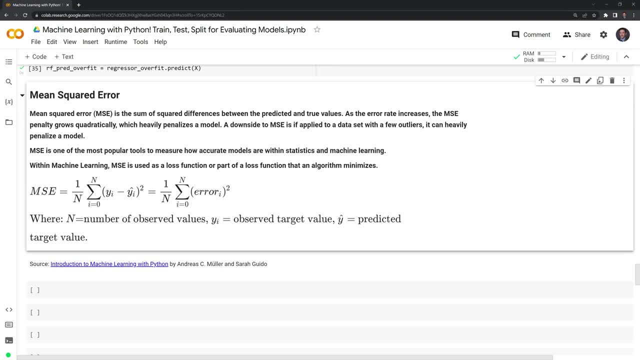 Training, 25% testing. The way that we can test our models is with mean squared error, And what this does is it takes the error. For example, if we can have a error of 100, or if we have a actual price of 100, a predicted price of 80, what we'll do is we'll take the 100 minus. 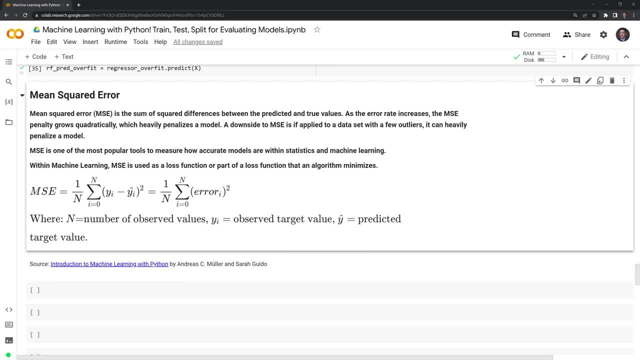 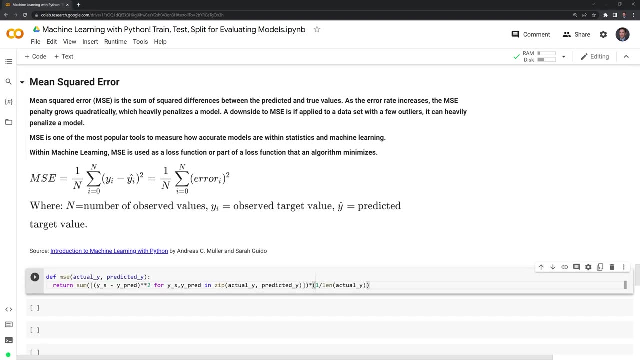 80, and then we'll square it And that's our error. We'll do that for each of the predictive values. we're going to get the error And we're going to sum over that and multiply it by one over the number of total values, And I have a function defined here that already does that for us. So I am. 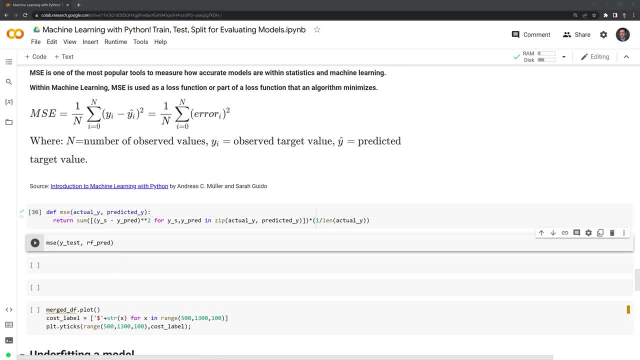 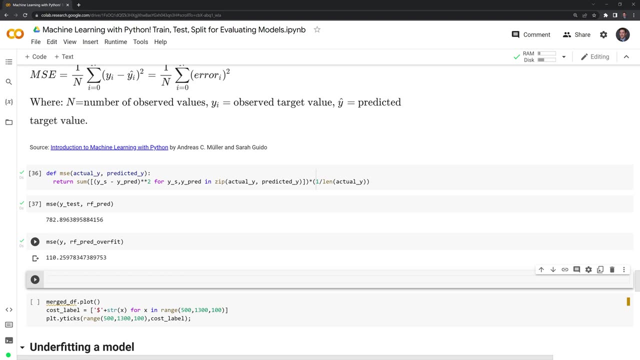 going to run that And I'm going to test both of the random forest prediction: the first, the one that was split 75%, 25% for training and testing, and then the overfit, And we can see that the one that was overfit is doing better And that's because that it was fed more. 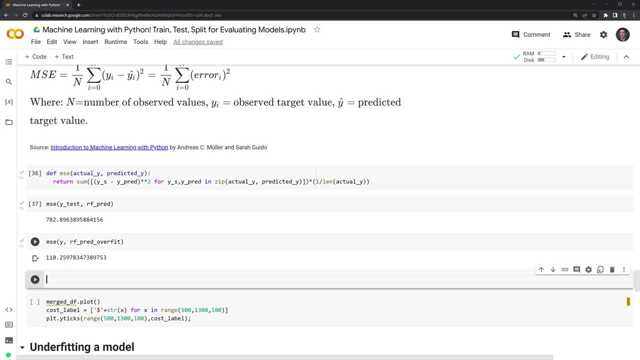 data. But just because the mean squared error is lower doesn't mean that it's better at predicting generalized data. This is predicting the just the sample data, The one where we split up. the training and testing data did worse, but it's more robust because we did this correctly. 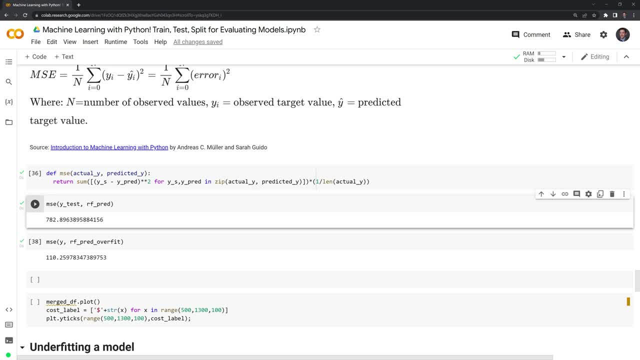 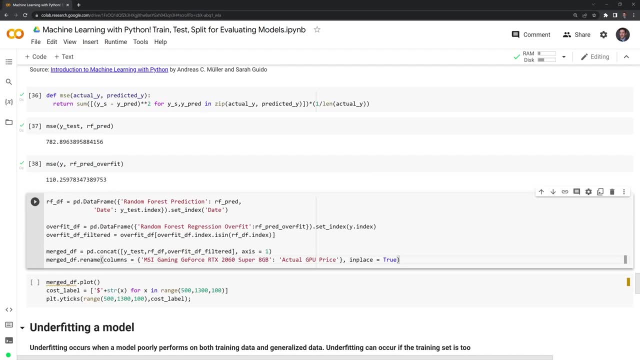 And we'll take a look at this even further. So what I'm going to do is I am going to plot this out And I'm going to save both the overfit data and the 75 25% data into a pandas data frame. what I'll 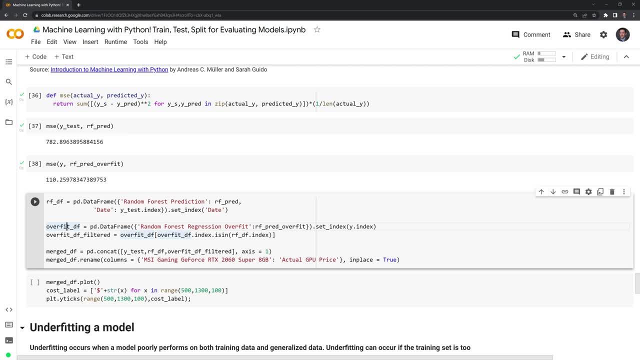 do is I am going to for the overfit. we're going to have more data points, So I need to filter down. the way that I'll do that is I'm going to call this overfit and I'm going to kill that calling this. 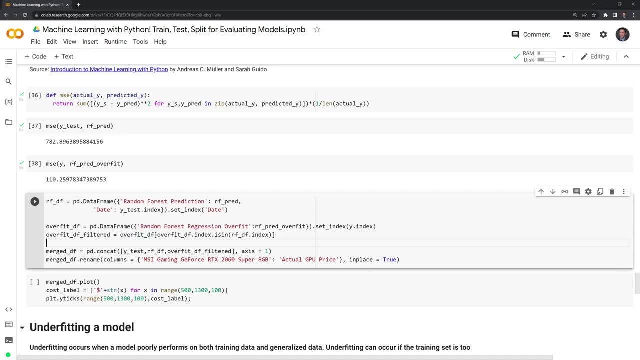 overfit And then within here I'm going to say based on the index, so we can get the date. if the random forest model from the first one contains a value will filter down to just those values. then we'll have this merged data frame which will plot out. So let's run this And then 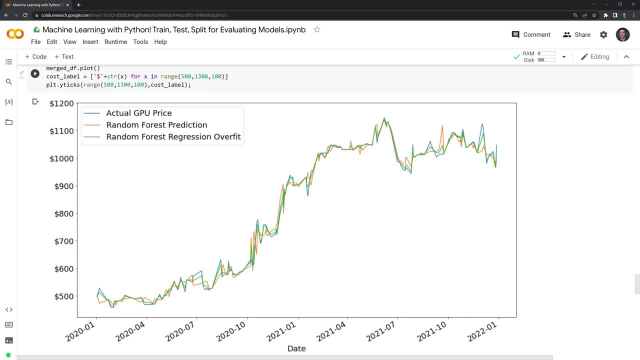 let's take a look at the plot. The blue line is the actual GPU price for the 2060.. We can see it here. it's very volatile as it moves up and down. The green is the overfit regression And we can. 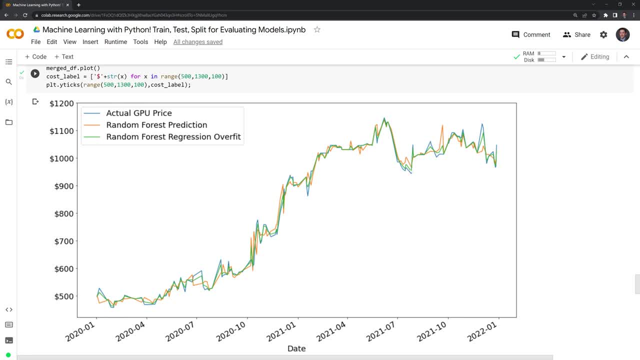 see that it's a lot closer to the actual data, But again, that doesn't mean that it was better at forecasting it. it just means that it was overfit because so many of all the data set was used in order to train that model, And we can see that for just the one that used the 75%, 25%. 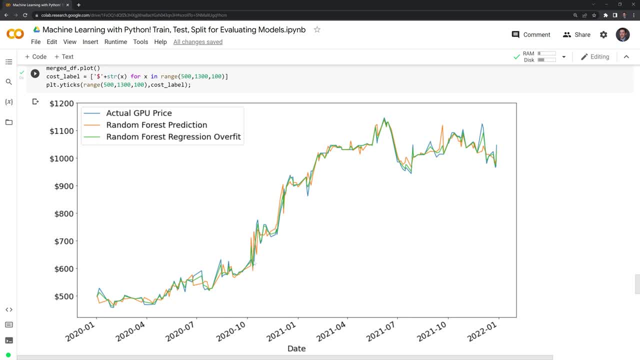 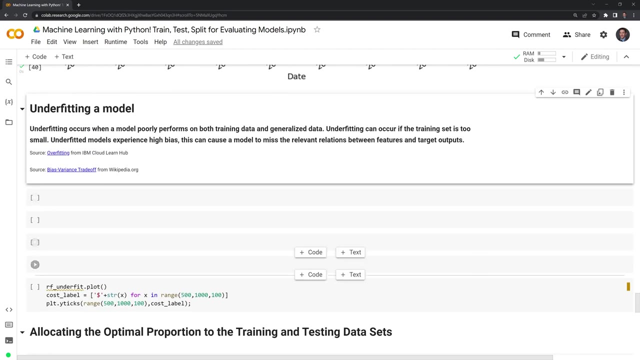 that's the orange. It doesn't match up quite as well relative to the actual price, And we'll see a further example of this as we go to look at the bias bias variance trade off later in the video. Next we're going to take a look at an underfit model, And underfitting occurs when a model poorly performs. 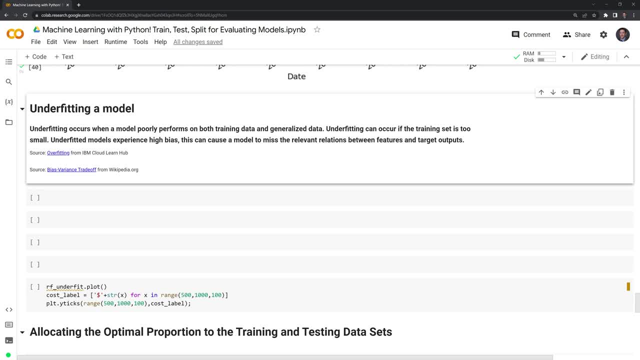 on both training at training data and generalized data. underfitting can occur if the training set is too small. Underfitted models experience high bias. this can cause a model to miss the relevant relations between features and target outputs. So what I'll do first is I'm going to create a small data set. 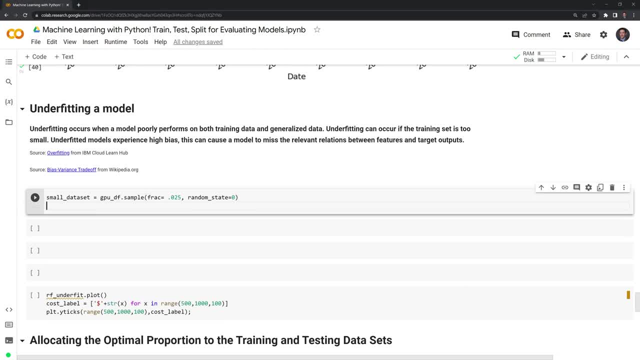 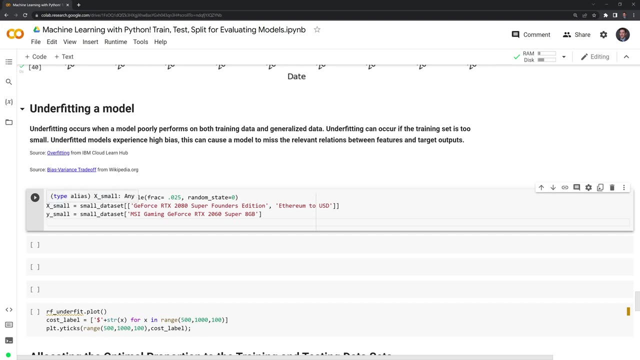 And in this case I am going to create the small data set by using the sample function again, but this time I'm going to get just a small fraction of the data. Then, after that, I'm going to create a PANDAS data frame for the explanatory variables and a panda series for the 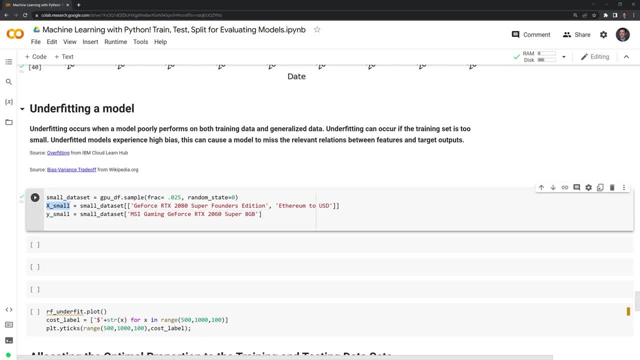 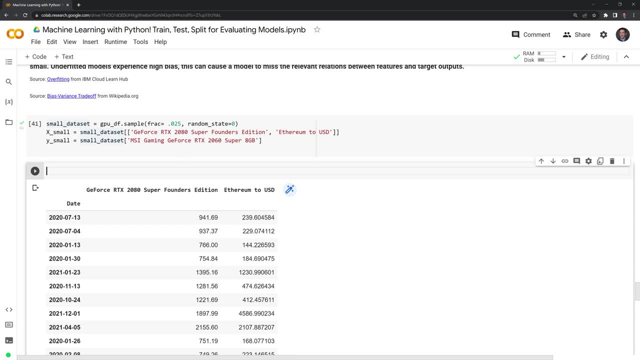 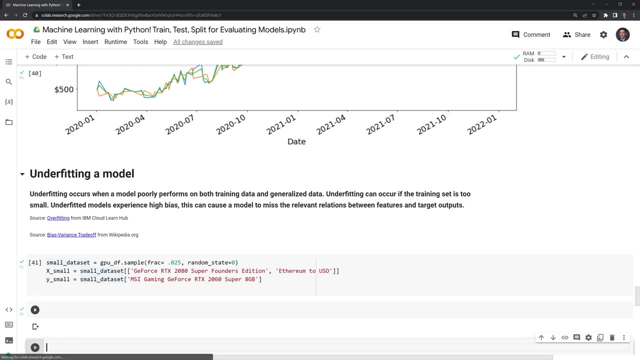 response variable. So we can take a look at one of the data frames and we can see we do not have a lot of points here. In fact, we only have 18 data points in all. So this is too small in order for us to be able to. 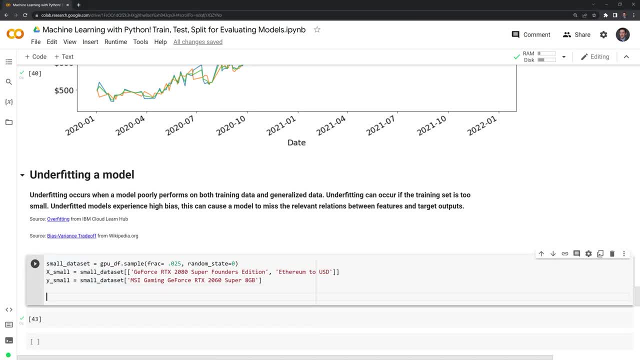 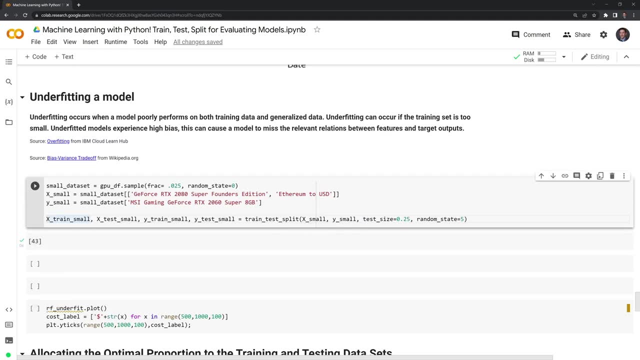 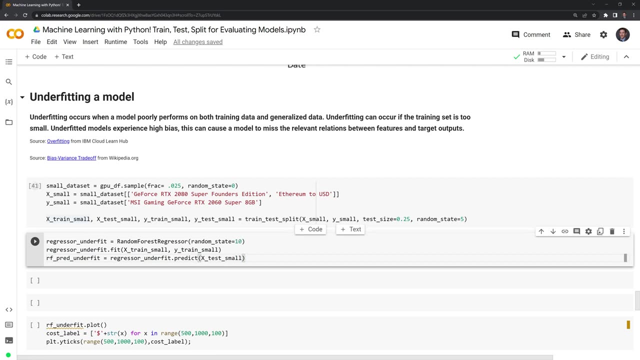 reliably model and we'll see the issues that comes with this. we're also going to split this into training testing data And we'll keep the same parameters as we did last time And, like before, we're going to create a model for the random forest based on. 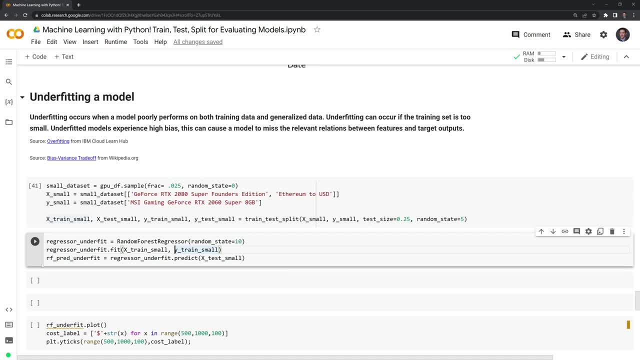 this small data set And we'll call this prediction random forest prediction under fit. we'll run this And what we can do is we could take a look at the mean squared error for this And we can see that it's really high relative to the two other models that we tried out, And 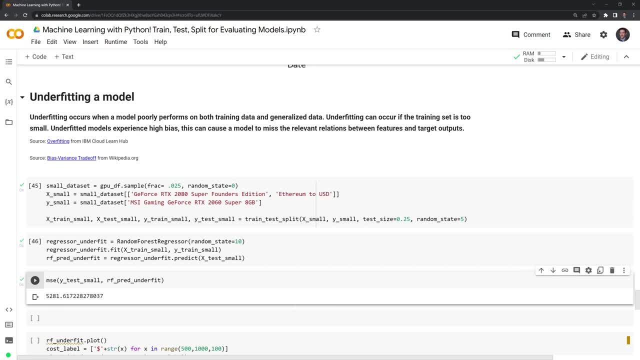 this is just because the data set is too small, It's under fit and it doesn't do a good job in predicting the data. I'll create a another data frame So we can actually plot this out and take a look at what it looks like And we can see here. 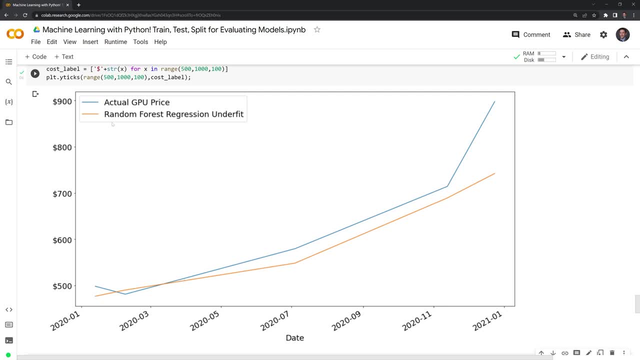 that it did not do a good job. we have: the orange line is our prediction And the blue line is the actual price. we can see that it's off by a significant amount. way out in January doesn't do as awful of a job, But still the because this is under fit. there's not enough. 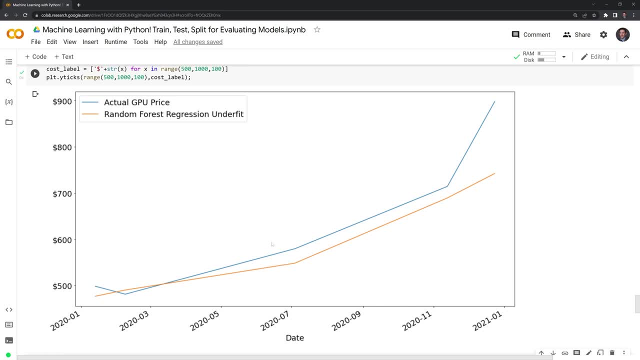 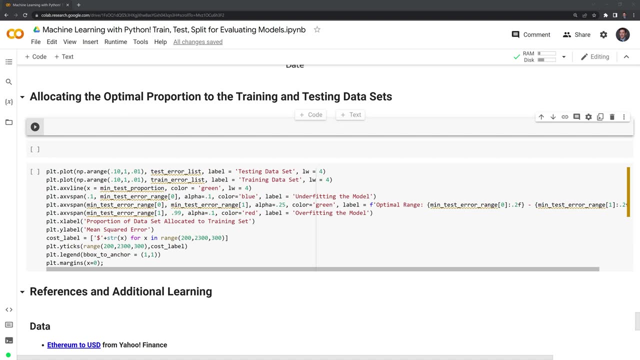 data. it doesn't do a good job in predicting what will the prices for the GPU. Next we're going to look at the optimal proportion to split the training and testing data sets. We'll have to do this with a for loop And we'll have to find the point at which the 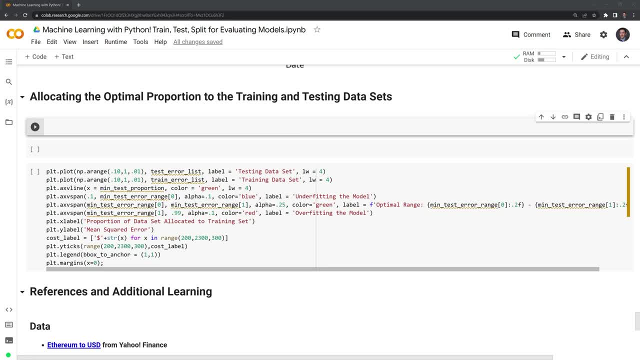 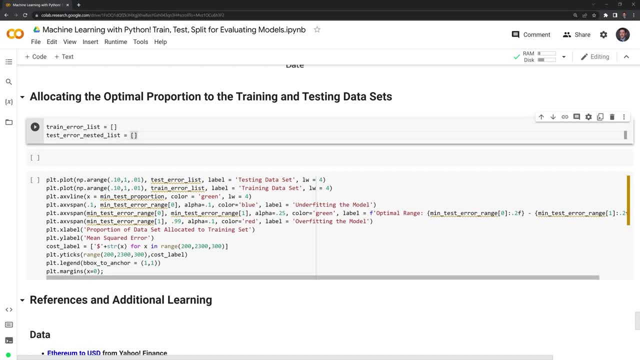 testing data set has the lowest mean squared error for our model. What I'll do first is I'm going to create two lists. The first is going to be a call a train error list And the the next is going to be the test error nested list, And I'll explain why that is. Then I'll go to the test error nested. 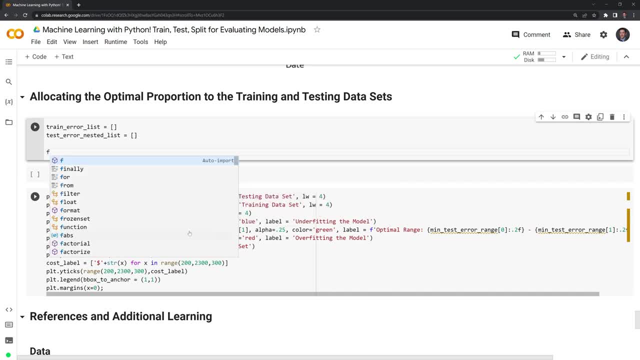 list And I'll explain why that is. Then I'll go to the test error nested list And I'll explain what this is later. Next, what I'm going to say is for I in np dot arrange And this is going to. 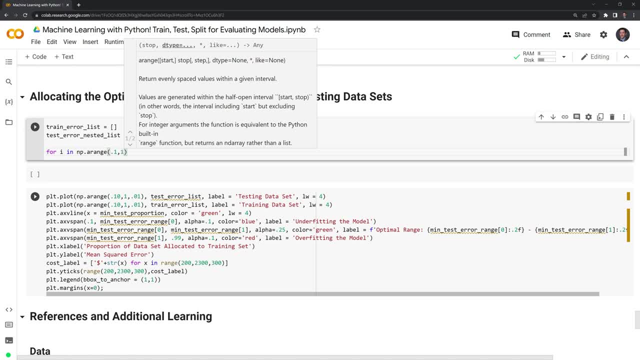 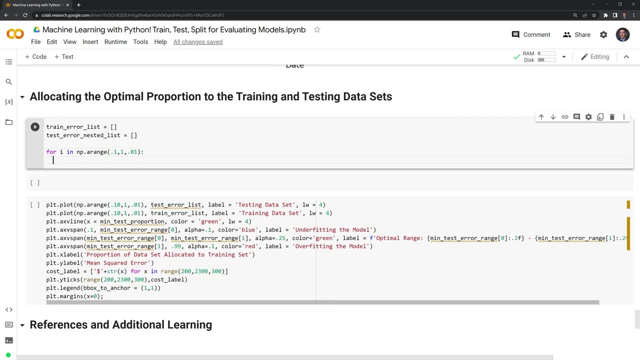 range from point one up to, but not including one. So it's going to go up to point nine. nine, because our step function is going to be point oh one, And what we're going to vary is the training size of our data set. So what I'll do next is I'm going to give in the x and y I'm going to create. 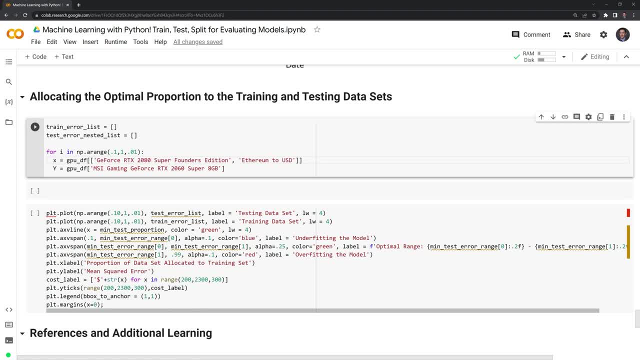 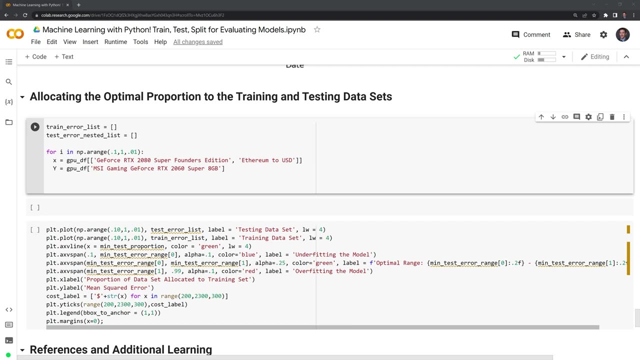 eight, two values, and I'm going to invert these, So lowercase x, uppercase y, because we already defined an uppercase x and lowercase y. Then next, what I'm going to do is, as the loop goes through, I am going to split the data. 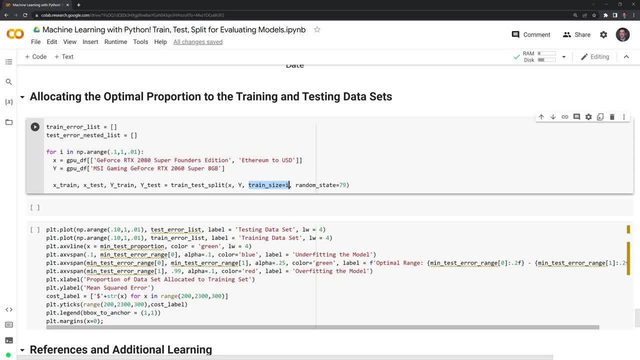 The only difference is going to be the training data set size. So at the very beginning, the training data set is only going to be test 10%, while the testing data set is going to be 90% of the data. all the way down to where the training data set is going to be 99% of the data. 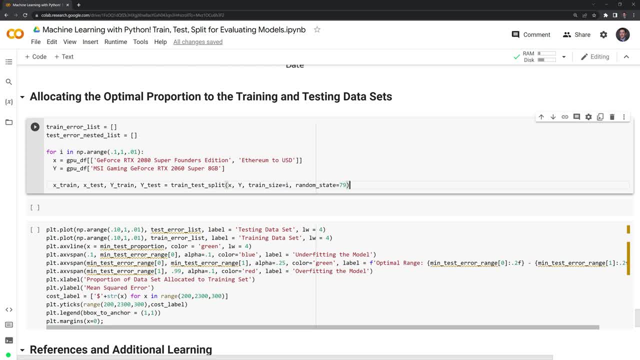 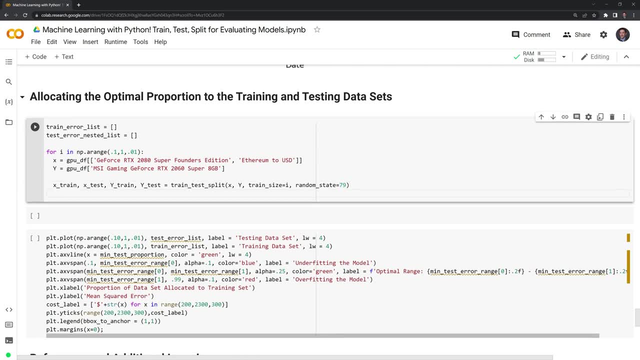 and the testing data set is only going to be 1% of the data, And we're going to seed it at a random state of 79,, just so we can recreate this. Then what I'm going to do is I'm going to set the training data set to 99, and I'm going to 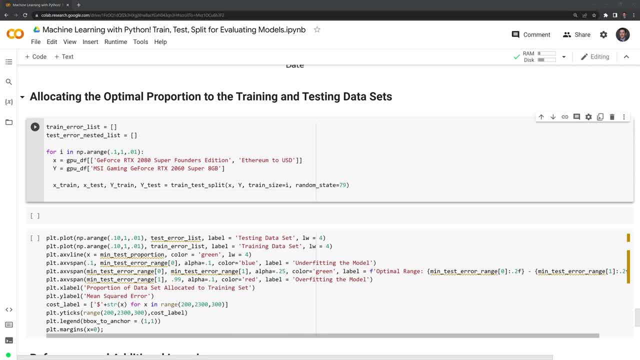 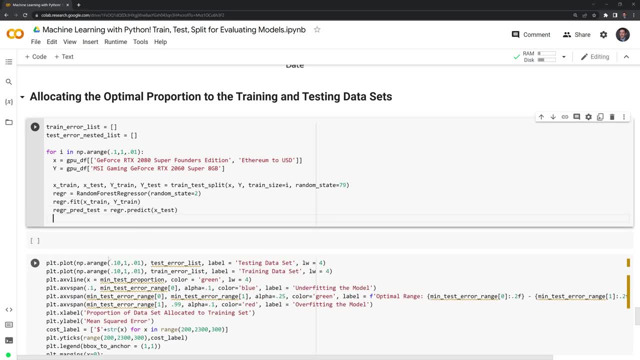 create a test error nested list. And what I'll do next is I am actually going to fit and train the models And this is going to be the random parse regression And we'll predict the values of the X test data And then, finally, this is where we save the data, So I'm going to call the test error. 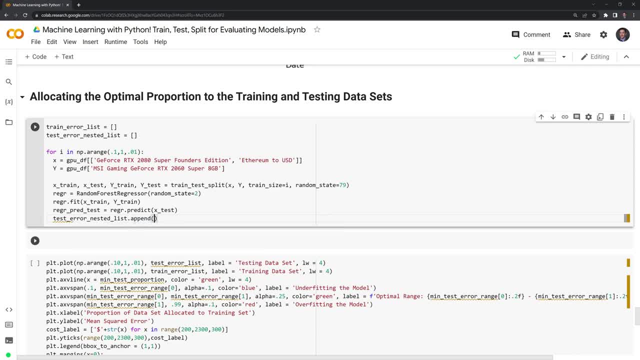 nested list, And what I'm going to append is going to be the mean squared error of the Y test and the X test, And then I'm going to set the test error nested list to 99.. And then I'm going to set the 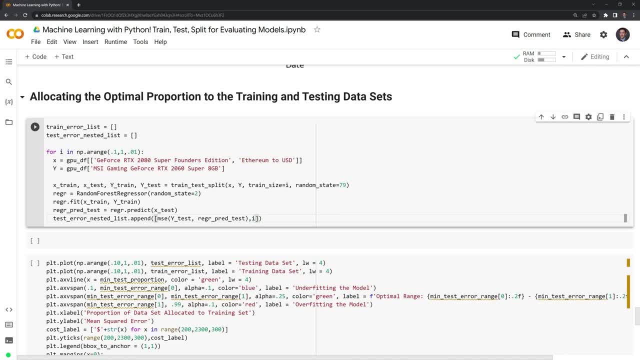 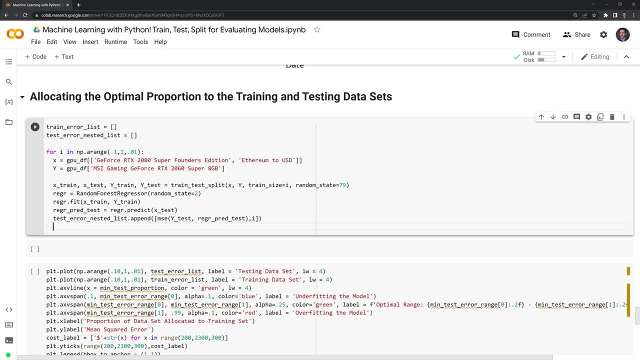 test error nested list to 99. And then I'm going to set the test error nested list to 99. And I also want to append the proportion. So this is going to be the proportion of the data for the training data set. Then what I also want to do is I want to predict on the extra X training data set. So I'll do that. 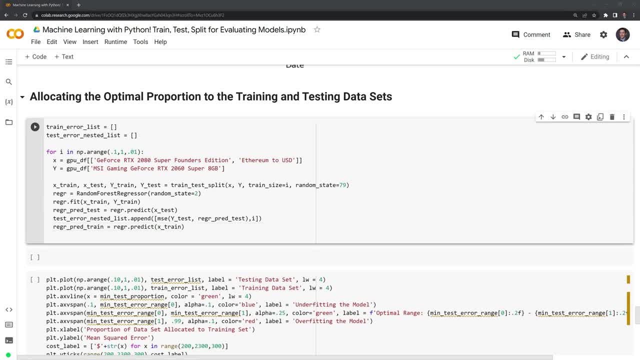 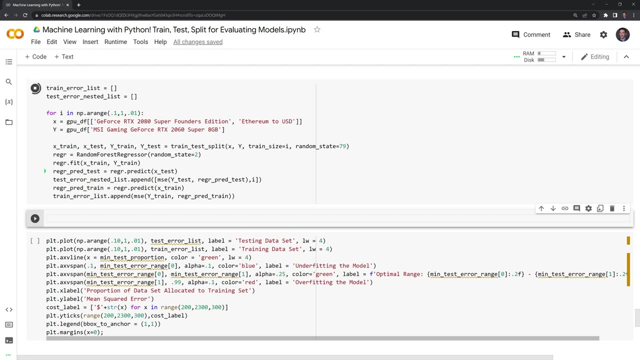 as well, And what I'll do is I am going to append all of these mean squared error values into the train error list That'll go through, So we can run this now, And this may take a few seconds because it needs to fit And for random. 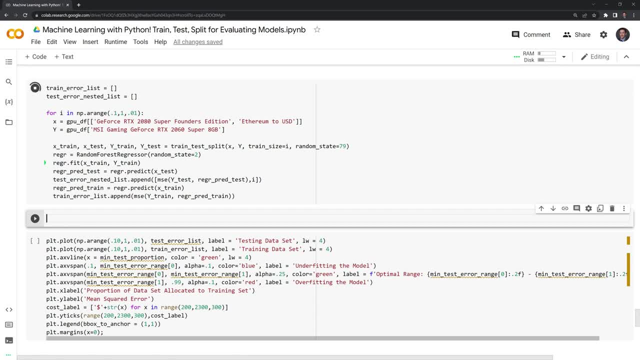 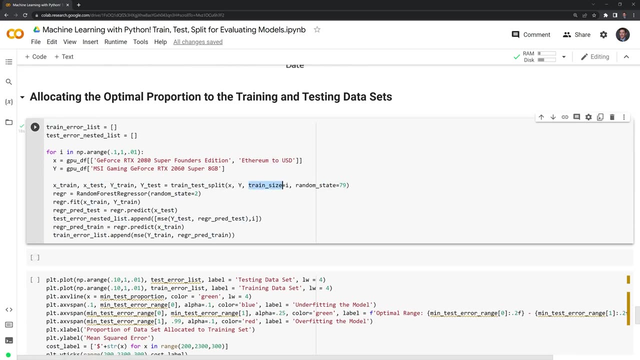 forests. it needs to fit a lot of decision. it needs to average across a lot of decision trees. Okay, so what I wanted to do first is I want to find the proportion of the data set, So the for what proportion of the training size, or what proportion of the training size? 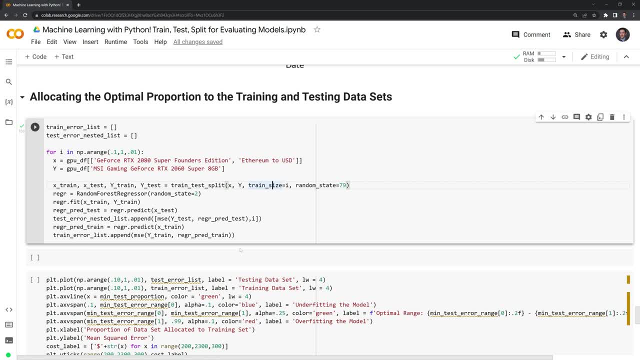 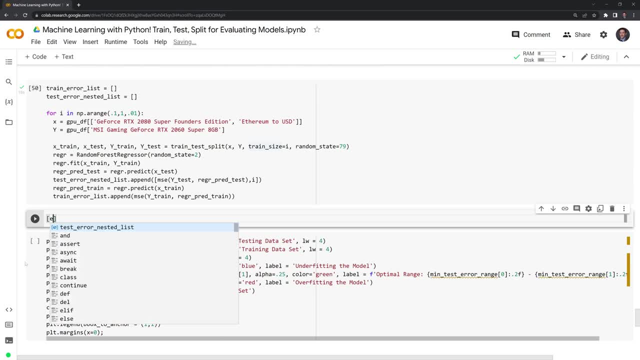 and then I'm going to do the test error nested list. So what I'm going to do first is I am going to use some list comprehension So we have a nested list. So what I'm going to say is error and then index position zero for error in test- error nested list. Let's run that. So I have a. 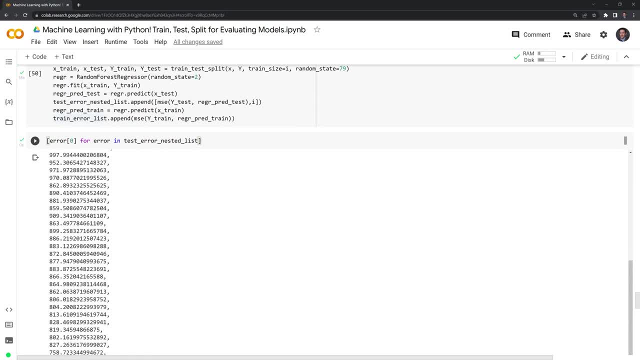 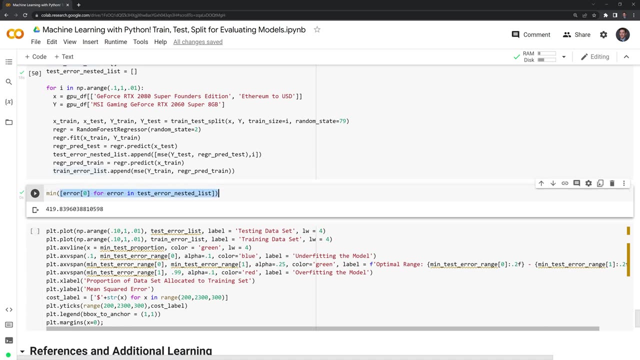 nested list of all the mean squared errors for the testing, And I want to find the minimum position for this. So let's run it, Let's see things, We can find the minimum numbers And then we can find the MN. what I'll do is I'm going to take this: 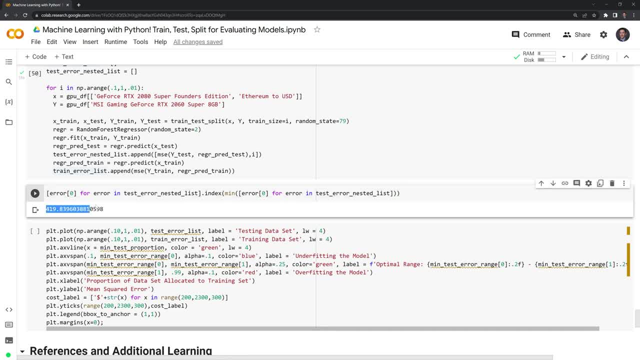 list and I'm going to say dot index And once we pass that value we'll get the index position for where this error is located. So let's run that. Hey, um, lowest for the test. I'm going to save this into a variable called min ID x and minimum index. 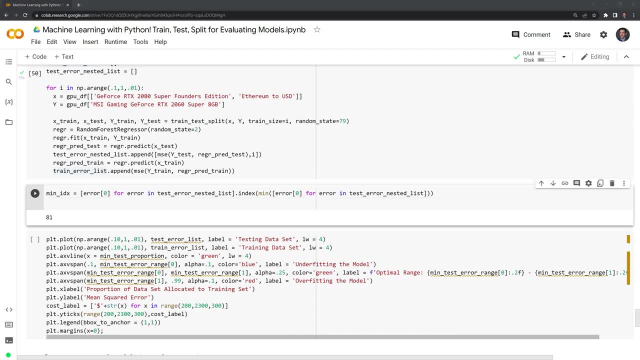 What I'll do next is I'm going to actually return the minimum test proportion. So I'll say test error nested list. Then what I want to do is I want to return the minimum index- Let's run that, So we have that, and I want to grab this value here. So this is the proportion where the training 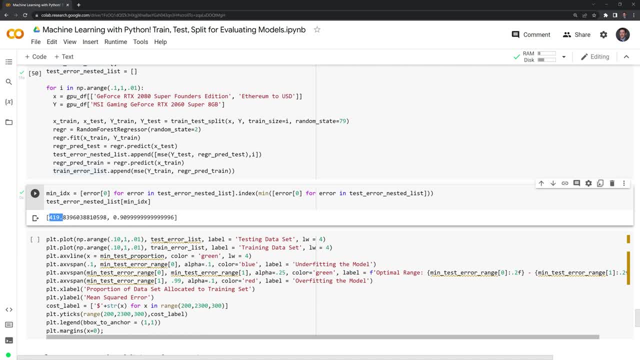 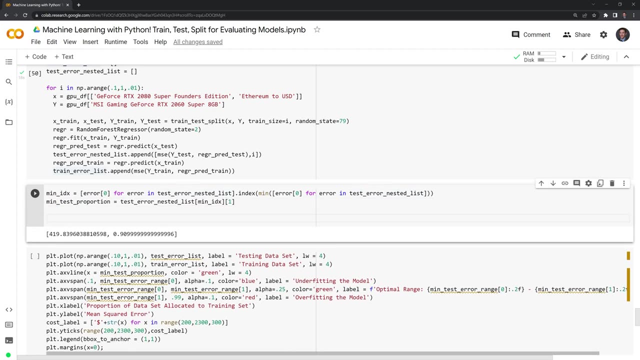 data set size optimizes for the best mean squared error, And I'm going to get this at index position one And we'll say that this we'll call this minimum test proportion. Next, what I want to do is I want to define a minimum range. So 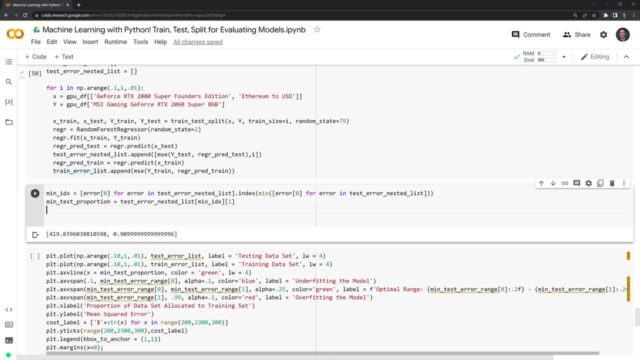 this is a single data point But in reality we probably have a range of proportions that are best for the training test size. So I could just say arbitrarily somewhere up or below by 5% we'd have our ideal range to set our training set proportion. 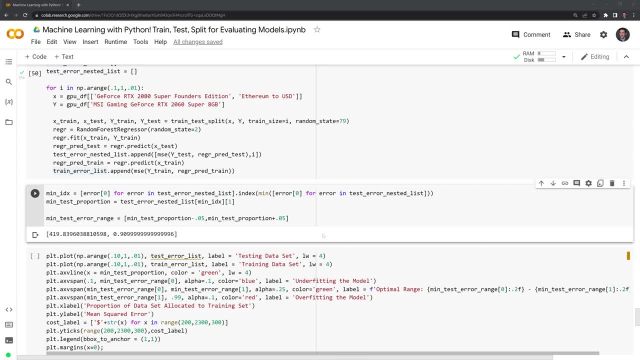 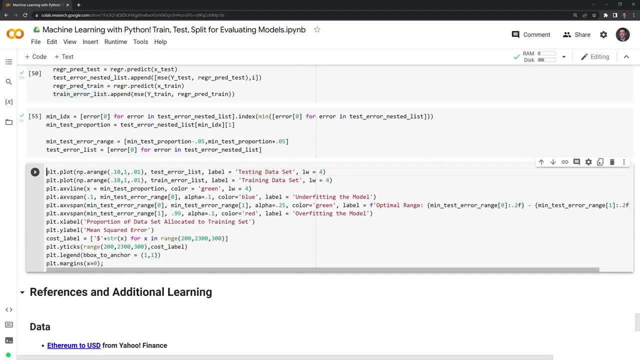 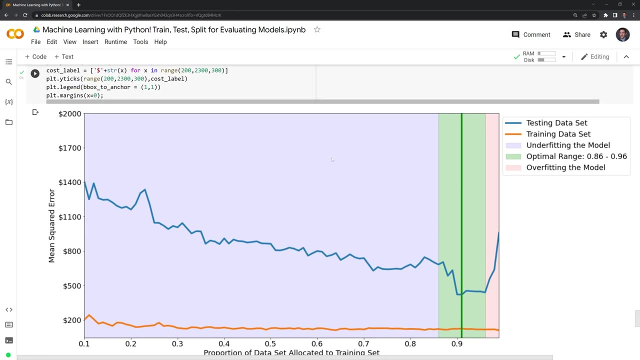 Then, finally, I want to save all the values And I'm going to unpack the nested list and save that. I over count And let's run this and take a look at our data. Great, And here we really have the. this summarizes pretty much everything I hope at. 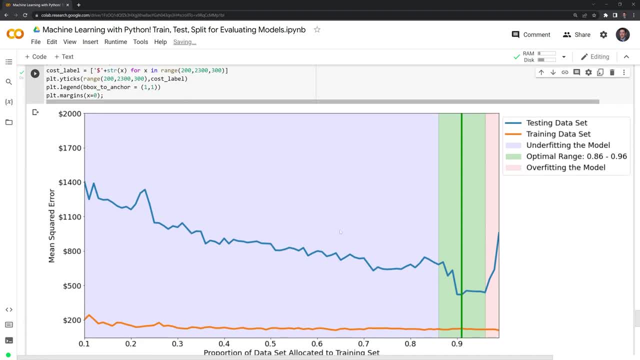 this point it will make sense. we had a lot of coding beforehand, But right here we have the testing data set And we can see that as we increase the proportion of data points going to the training data set, that the testing data set will beフ gosh. eleven percent, plus every training data set that the testing data set will는rode to a Iket and Array Dome dweltdisk, plus every training data set over the training data issay that the data isl as any number of times going to this is equal to e, thats when. so you get thatманipal does that and so attached all in. 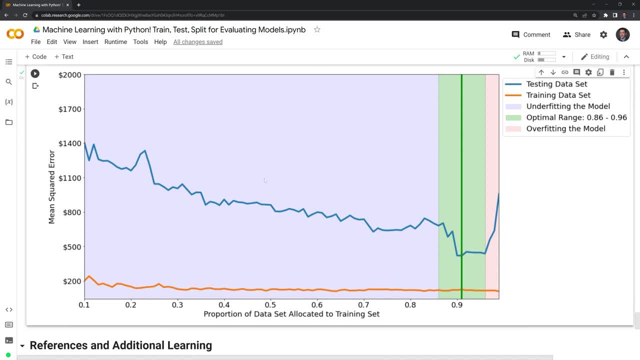 But when I'm parallel, assez tu marketers asauce work. as ifu can see, as we have a additionally low issues to common cause, the testing data set the mean squared error gets lower and lower. So that means our model is doing better, the lower the mean squared error. we can also see that the training data set the mean. 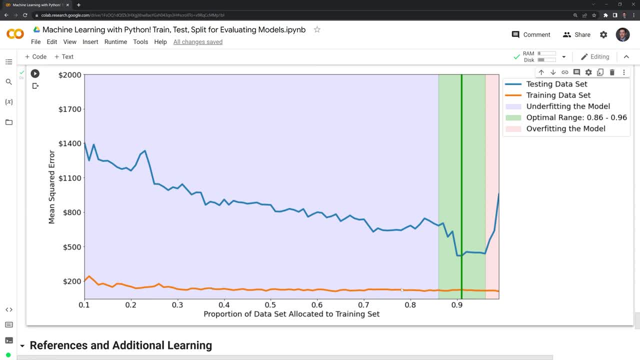 squared error continues to lower throughout. However, we reach an optimal point right around looks like 91%- where this is the point where, if we keep increasing the training size, then the testing data set, the mean squared error for a model, is going to increase. So we would want